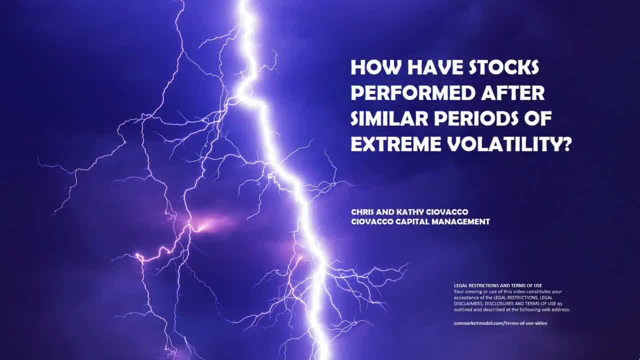 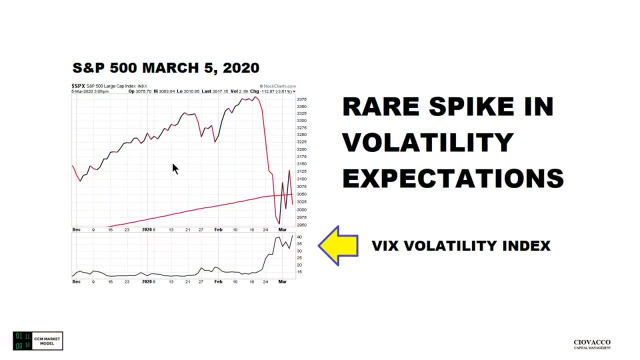 In this week's video, we take a detailed look at similar periods of extreme stock market volatility to get a better understanding of potential risk and reward walking forward. The top portion of the chart on your screen is a daily chart of the S&P 500 index as of March 5, 2020.. 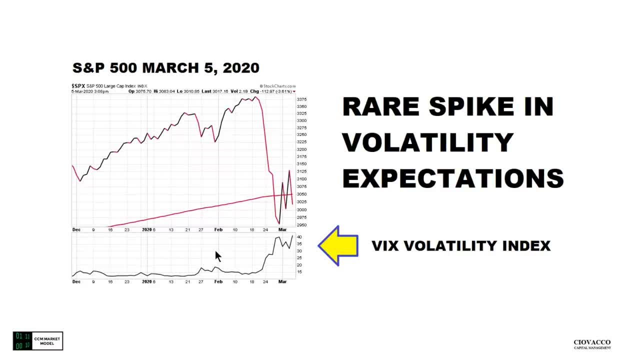 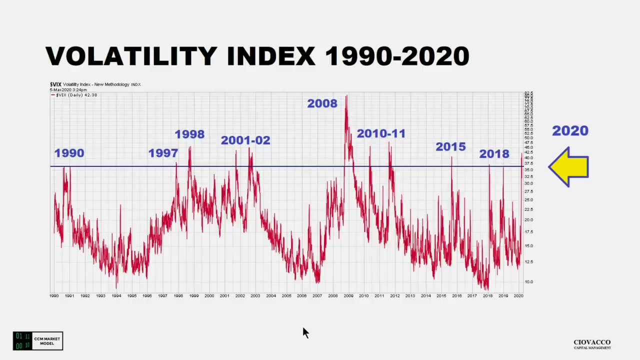 This is the 200-day moving average. Bottom portion of the chart is the volatility index, affectionately known as the VIX. This is a relatively rare spike in volatility expectations, which is a little bit easier to see if we look at a longer-term chart of the VIX. 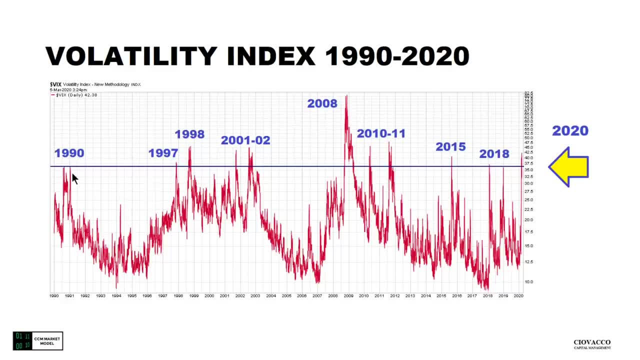 This is the recent spike here. This is calendar year 1990.. Why 1990?? We only have data going back to 1990.. You can see the giant spike here in volatility expectations in calendar year 2008.. An important caveat. 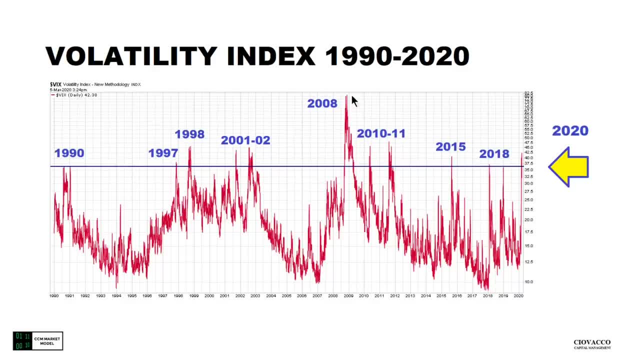 Before we begin, our study is based on a spike in volatility expectations, and the numbers that we're going to cover apply after the VIX has stopped rising. As of the close on Thursday, March 5,. the recent high was made. The spike in volatility expectations was made on Friday, February 28,. 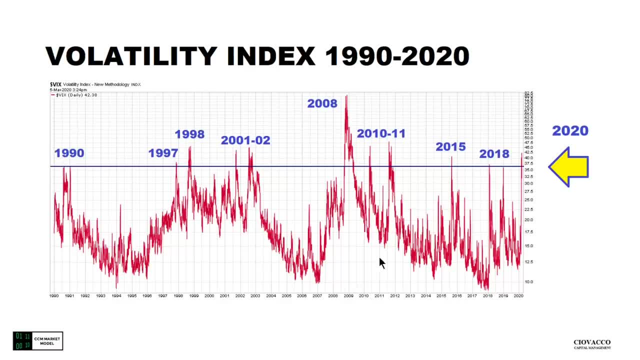 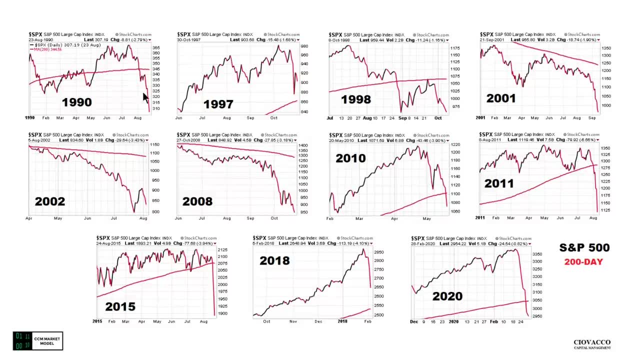 and that is our benchmark for this study. As you might imagine, a big spike in volatility expectations Often occurs during big plunges in the S&P 500.. These are the exact same dates. This time we're showing a chart of the S&P 500 index. 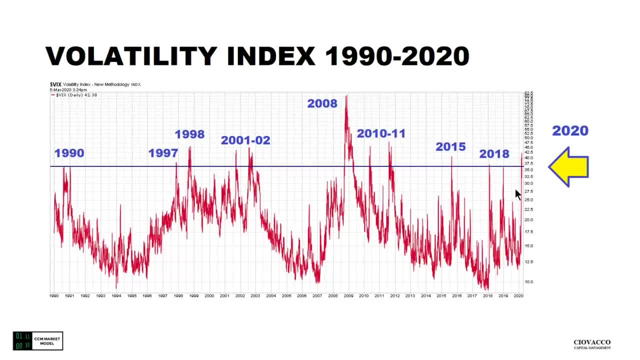 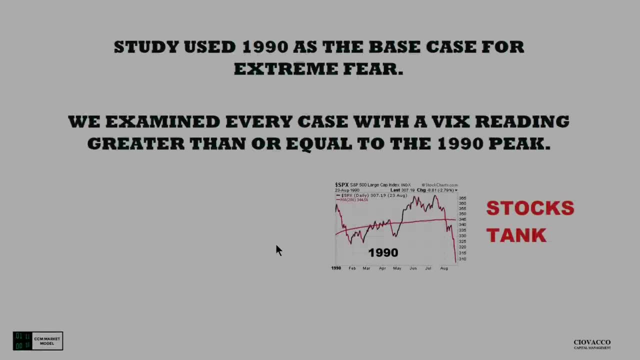 These are the same cases with the VIX. How rare is the spike that occurred on Friday February 28?? Only 10 previous instances dating back to 1990.. Since we want to study the most extreme spikes in volatility expectations, we used 1990 as the base case for this. 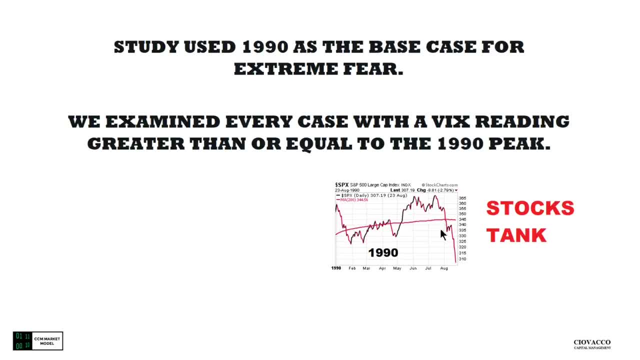 This is a very, very similar to the present day. in 1990, stock market tanks in a waterfall fashion and very, very similar to the present day, we get a big spike in the VIX or the volatility index And, as common sense would tell us, we don't get stock market plunges like this without some type of fundamental issue that the market is extremely concerned about. 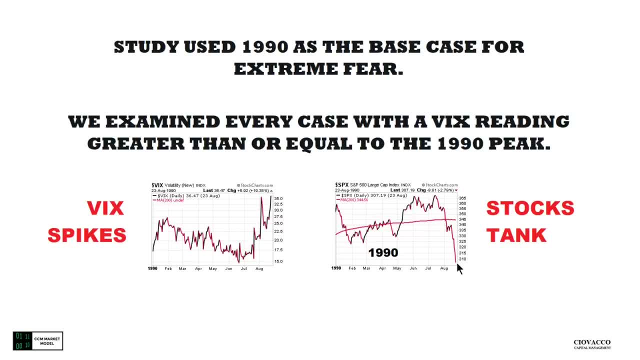 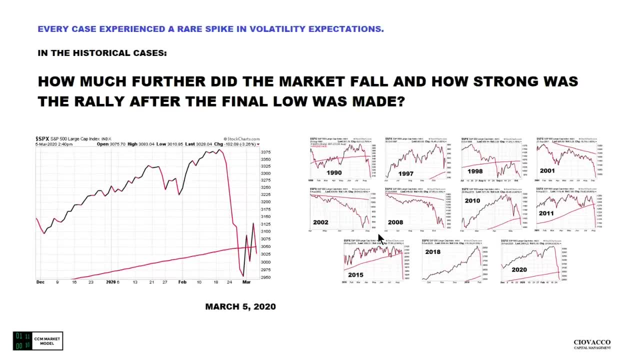 Thus, in the present day, it might be helpful to know what happened in this case, walking forward after the VIX reached a peak, and how much further did the stock market fall and how strong was the rally after the final low was made in the S&P 500.. 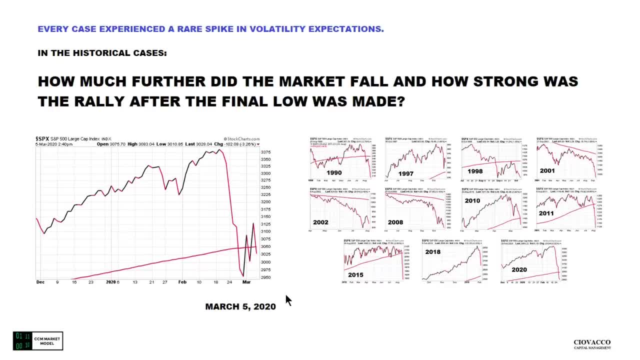 The answers to those questions will give us some reasonable expectation from a historical perspective as to how far the market could fall in 2020, when a bottom might be reached from a probability perspective, and what type of rally we could expect if a bottom is reached. 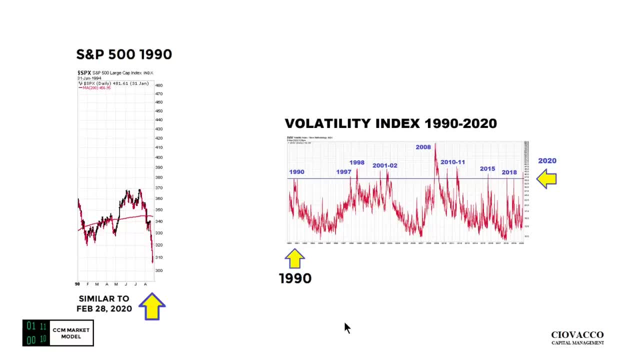 So let's walk through each case individually and see what we can learn, And then we will look at a summary of all the cases. S&P 500- left side of your screen, 1990.. This plunge here in the stock market is similar to the look in the stock market on February 28th 2020.. 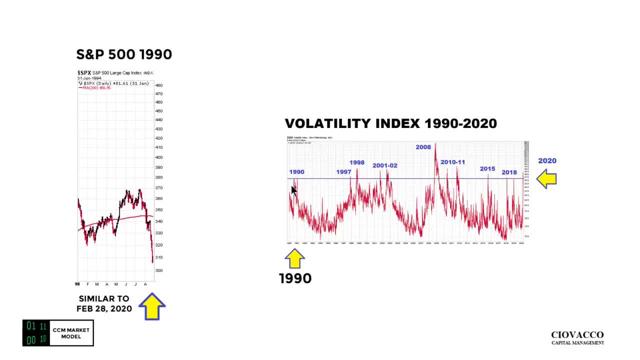 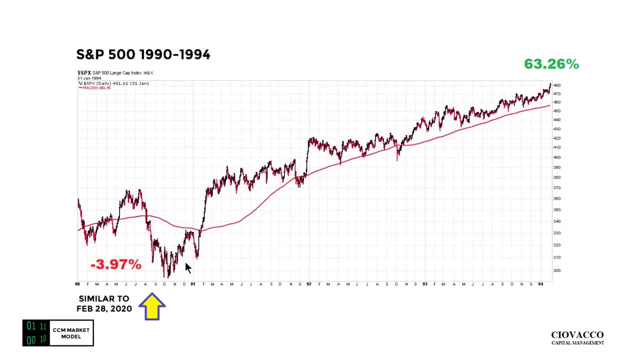 Present day case. Here's our spike in the VIX. Here's the similar spike in the VIX in calendar year 1990.. What happened walking forward from the date that is similar to Friday February 28th In this case, if you were able to withstand an incredible amount of gut-wrenching volatility, 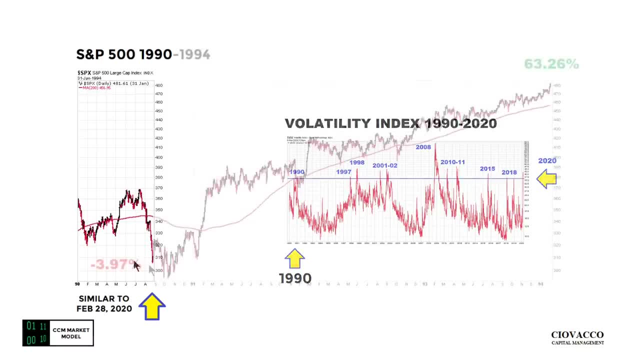 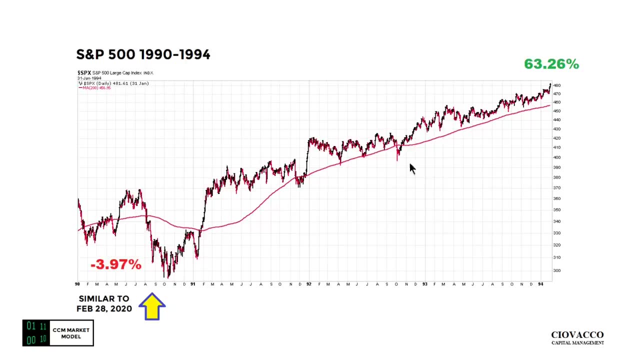 and you were able to withstand an additional drawdown of 3.97% from the day. that's similar to February 28th. really, good things happen. for a long period of time. From this low, the S&P 500 tacked on. 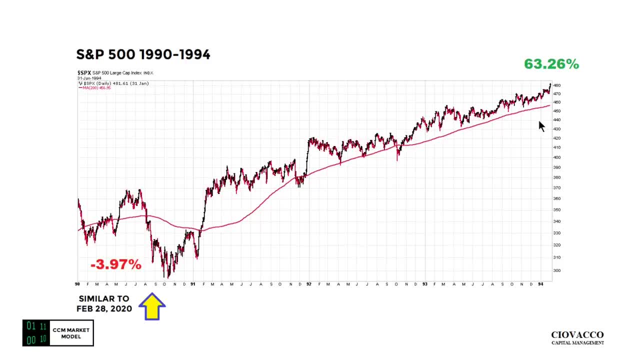 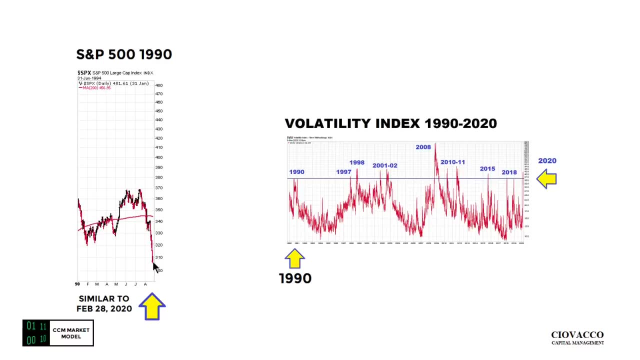 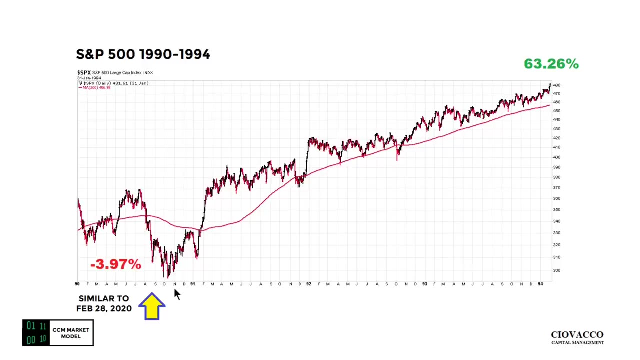 63.26%, and the rally did not end until early 1994.. The whole purpose of this study is to better understand historical risk, which in this case was an additional drawdown from the low of 3.97%, and historical reward. 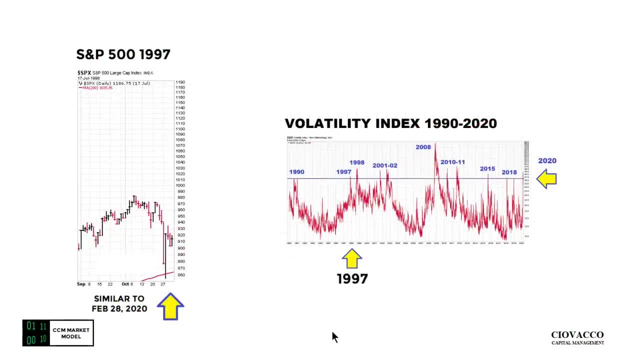 which in this case was a gain of over 60% Calendar year 1997.. I can assure you this plunge here was extremely uncomfortable. in real time We get the similar spike here in the VIX, similar to what happened in the present day. 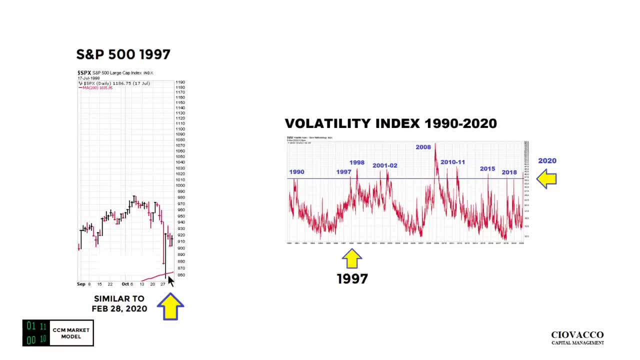 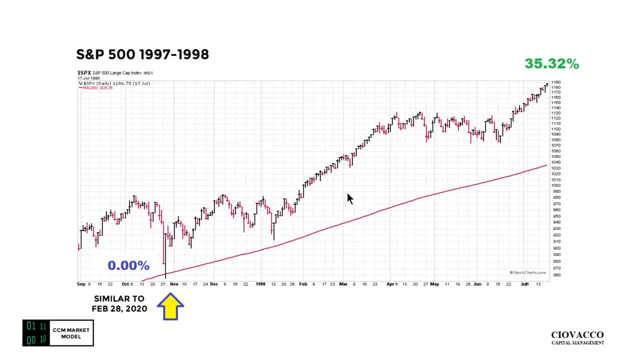 In this case, if we were able to remain cool, calm and collected when the market was plunging, that composure was rewarded in a big way. The S&P 500 gained 35.32%, And in this case, the spike in the VIX occurred on the same day that the S&P 500 bottomed. 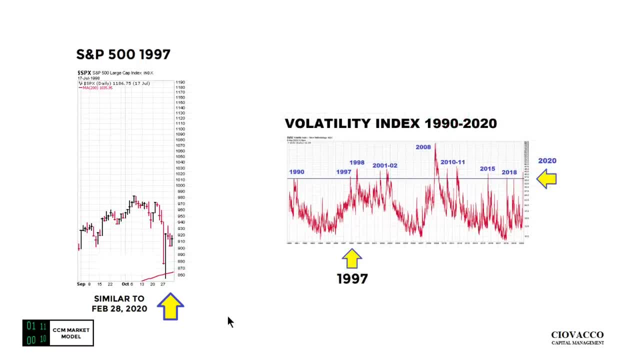 Thus, based on this historical case, it's within the realm of reason that the S&P 500 could have made a bottom on February 28th, And obviously that is to be determined. Kathy and I have been working on Wall Street since the 1990s. 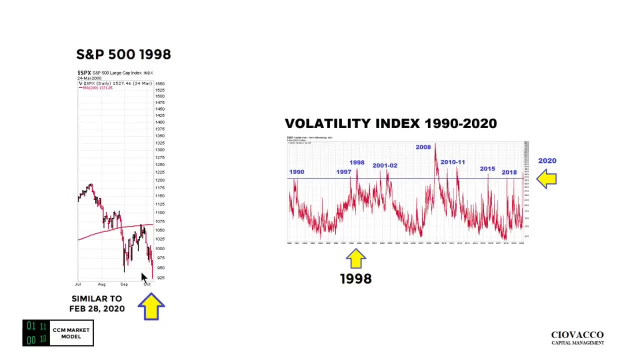 and we both can assure you that it was very, very uncomfortable to be anywhere near a screen during this period here in 1998.. From this point in October 1998, the VIX put in a high and then started to fall, If we were able to remain cool, calm and collected during this period. 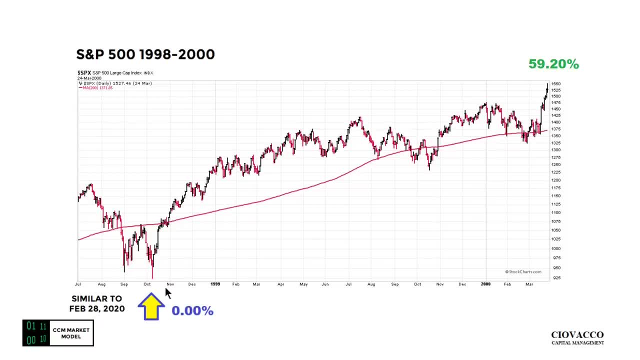 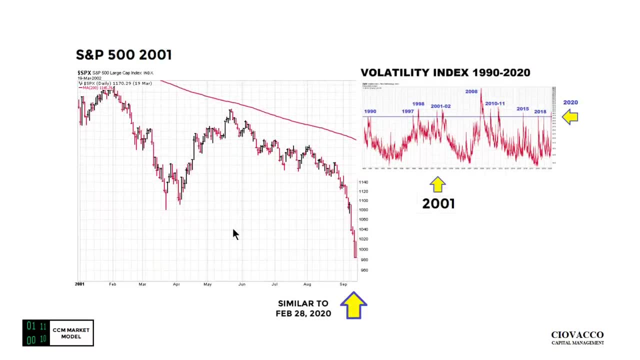 once again. that high in the VIX marked the end of the decline for the S&P 500. It righted itself and gained 59.2%. What happens if we're going into a bear market? Well, this example from history occurred during a bear market. 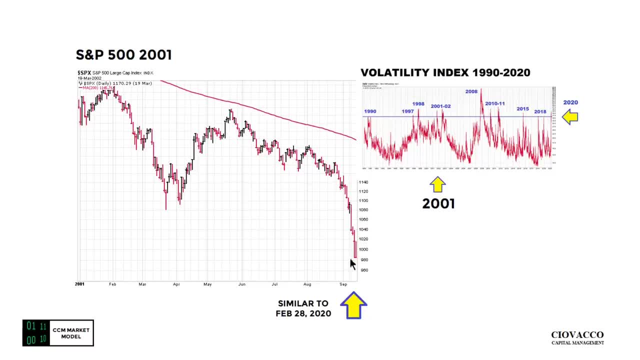 A very uncomfortable multi-month plunge in the S&P 500.. Big spike in the VIX and a reversal similar to the levels in the price range In the present day. what happened walking forward from this point? a point that occurred in the middle of a bear market? 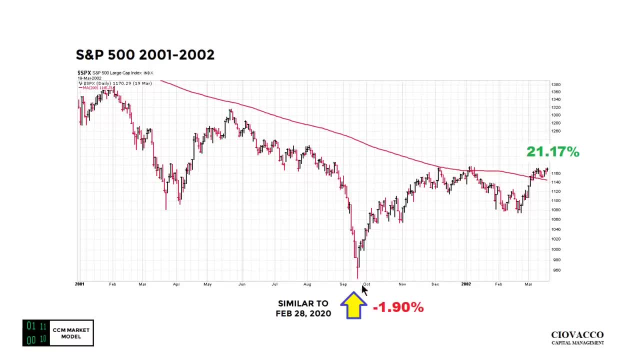 after this waterfall plunge here the market rallied from an extremely oversold condition, lost an additional 1.9% after the VIX spiked, but from that point it gained 21.17%, Telling us that, even in the context of a horrible bear market, that was not over yet. 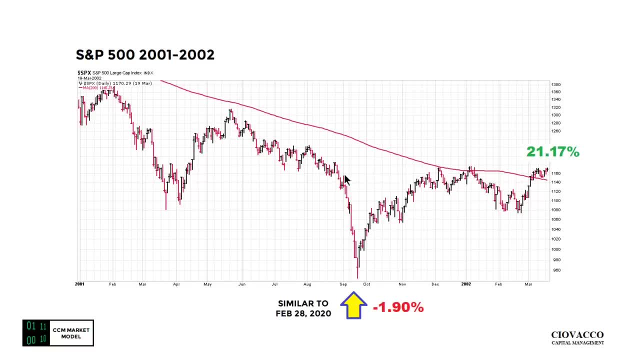 the extremely bear spike in fear and oversold condition of this market was followed by an extremely powerful rally. The purpose of our study here is to try to understand what we should be doing in the present day. From this low here to this high here, it took. 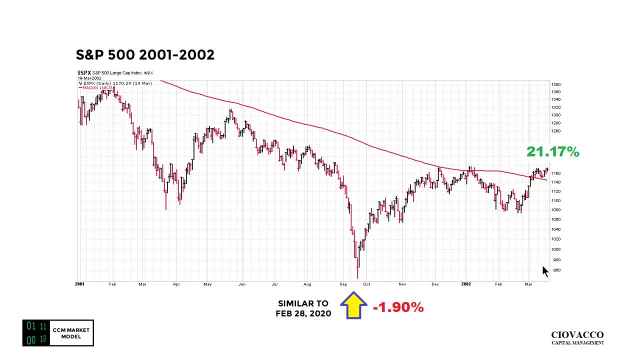 1,, 2,, 3,, 4,, 5,, 6 months, Telling us that, even in the context of a devastating bear market, patience from this type of condition in this case was rewarding. It was rewarding in a big way. 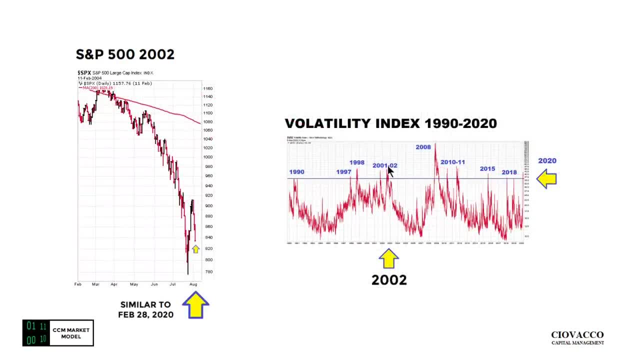 Fast forwarding to the 2002 spike in the VIX here. The VIX peaked here, which is similar to February 28th 2020, walking forward in the S&P 500.. Did it get better, worse or did it stay about the same? 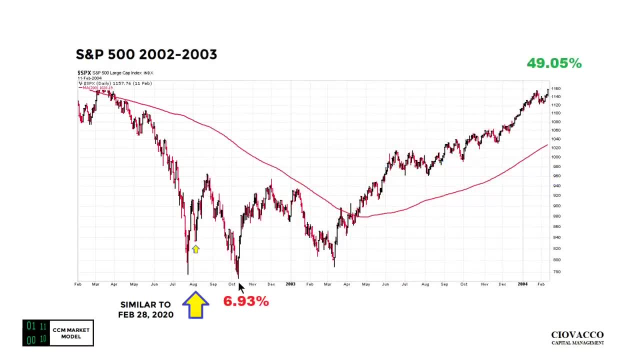 The original low was retested and notice here a retest of the low can exceed the prior low. This is still a retest of this low and this is a successful retest. The drawdown, additional drawdown from this point here, which is similar to February 28th, was almost 7%. 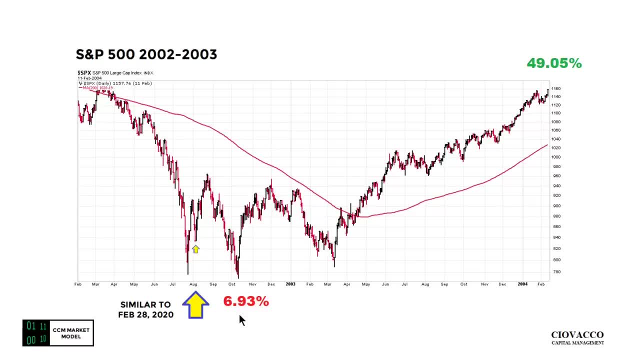 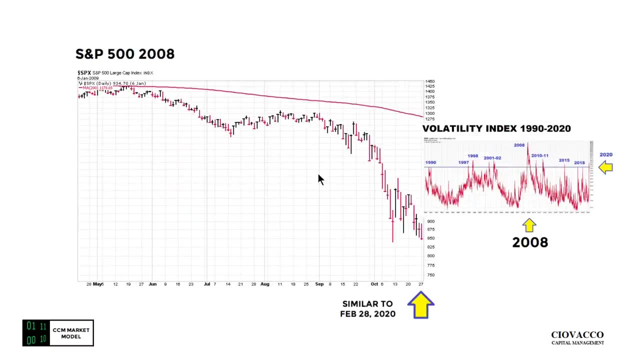 That's extremely painful, But for those that were able to navigate properly after the successful retest of the low, really good things happened for a long period of time, with the S&P 500 tacking on 49% plus. This 2008 case occurs during an extremely high period of fear. 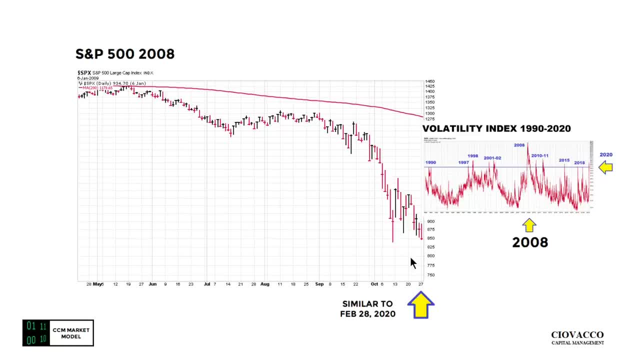 In Q4, of 2008, in the financial crisis. this is the day where the VIX stopped spiking and eventually reversed. It would be similar to February 28th if the VIX does not go on to make a higher high. 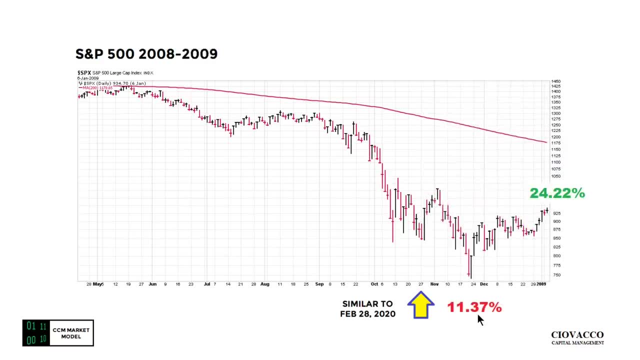 Walking forward from this point, the market lost an additional 11.37% but then rallied sharply 24.22% off of that low, Reiterating that typically rare spikes in volatility expectations and typically extremely oversold markets even from horrible technical profiles. 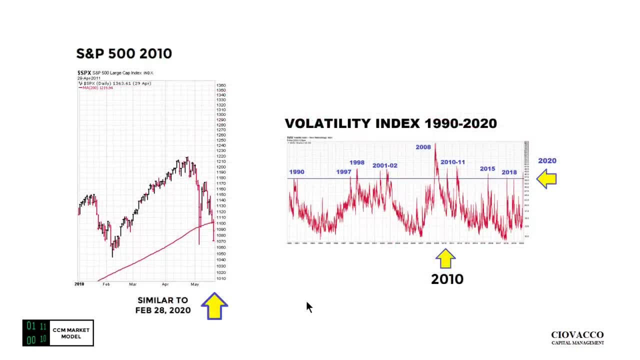 tend to bounce in a big way. 2010 case. it's been very, very uncomfortable in the present day. This was extremely uncomfortable in May of 2010.. Here's the spike here in the volatility index that is similar to the spike in the present day. 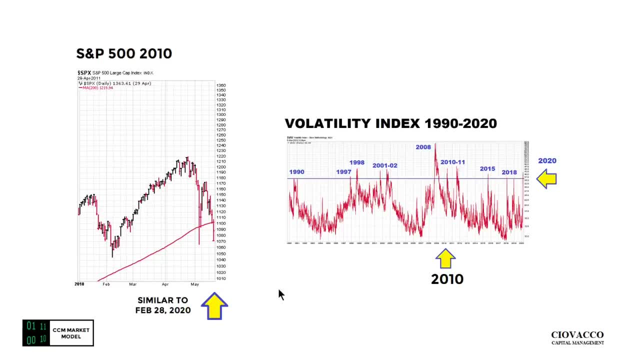 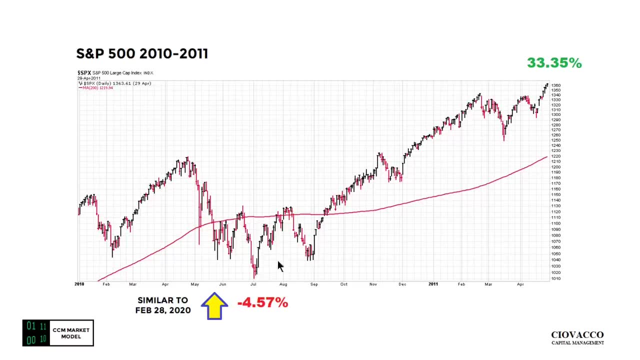 What happened walking forward in the S&P 500? Said many times that often a low is retested. Here's the first low: We rally, we come back. This is a form of a retest. The market holds in the general area and then rallies and puts in a bottoming formation. 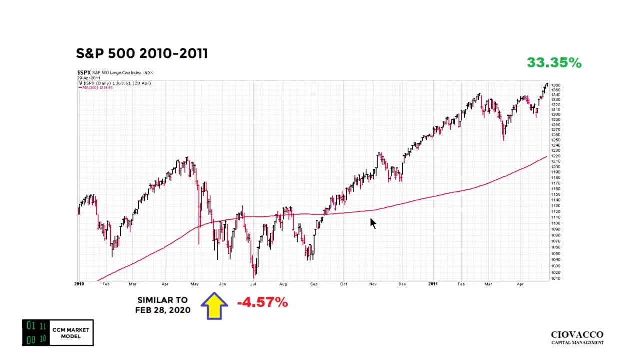 You can make an argument. This is an inverse head and shoulders pattern. For those that didn't overreact in this area, here they were rewarded with a 33.35% gain in the S&P 500.. For those that didn't overreact in this area, here they were rewarded with a 33.35% gain in the S&P 500.. They were rewarded with a 33.35% gain in the S&P 500.. They were rewarded with a 33.35% gain in the S&P 500.. 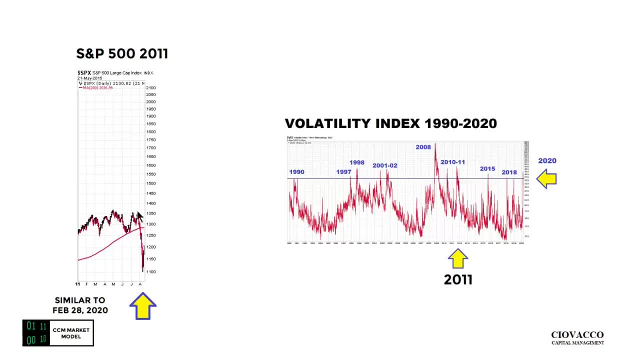 In the subsequent months. A lot of similarities between the plunge in 2011 and the plunge that we're experiencing in 2020.. A lot of differences as well. This formation prior to the plunge is quite a bit different than walking into the plunge in 2020 and 2019.. 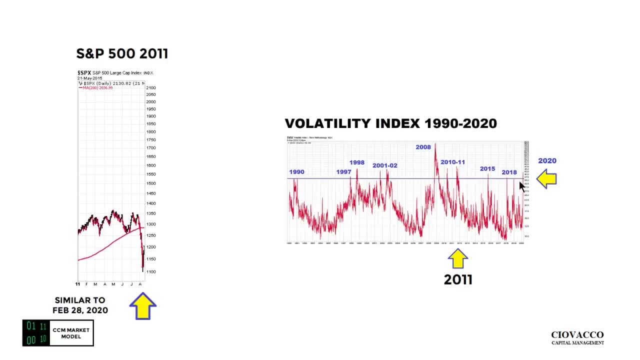 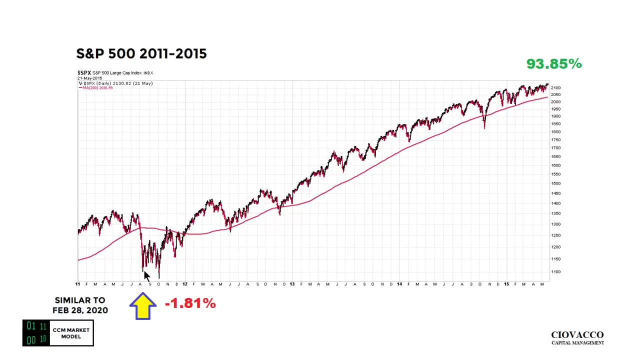 We still have a very similar move in the VIX calendar year, 2011-2020.. Walking forward in the S&P 500.. What happened? A lot of volatility- Sound familiar. Eventually, we retested this low In this case. 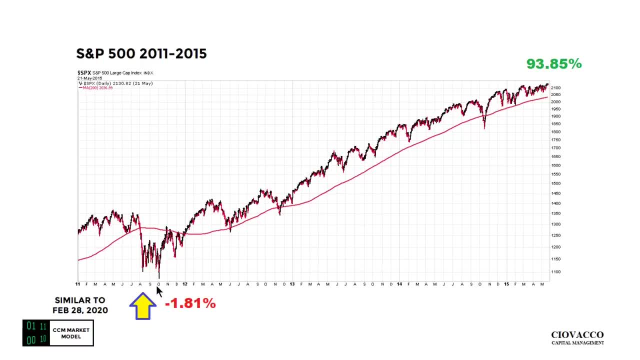 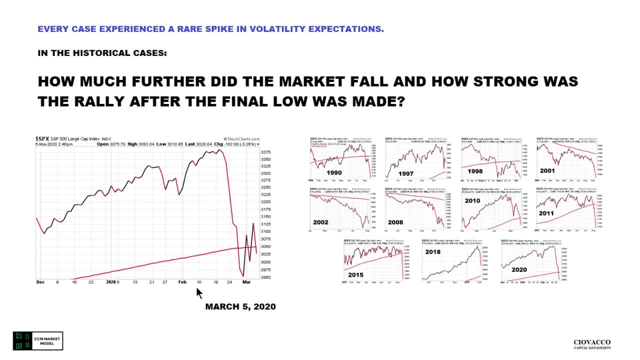 the retest, we made a lower low. That's perfectly acceptable for a retest, which means in the present day, if the S&P 500 exceeds this low here from late February, it doesn't mean the retest has failed, Walking forward in the 2011 case. 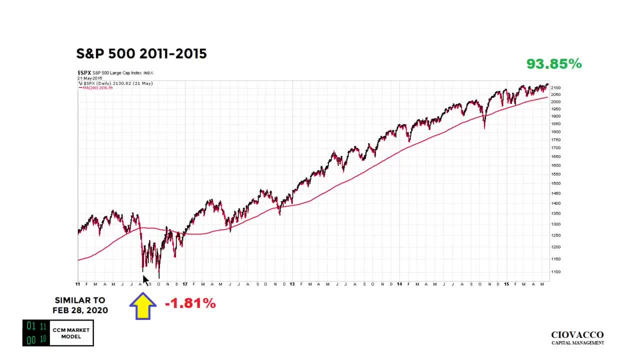 we dropped 1.81% below this low here, And then from an extremely oversold condition and after a big spike in volatility expectations similar to what we've recently experienced, patience and composure was rewarded in a big, big way. 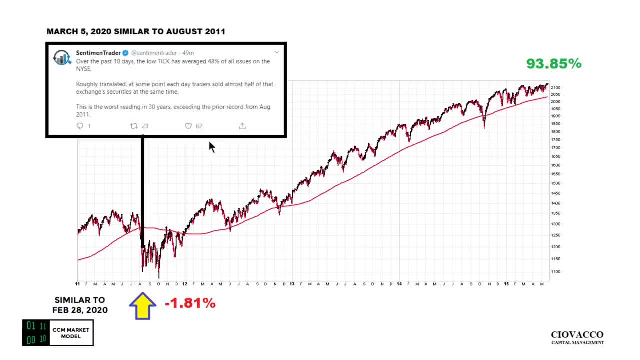 We started working on this study earlier this week. Then another piece of evidence came to light during the week from sentiment trader Thursday of this week. over the past 10 days, the low tick has averaged 48% of all issues on the MYL. 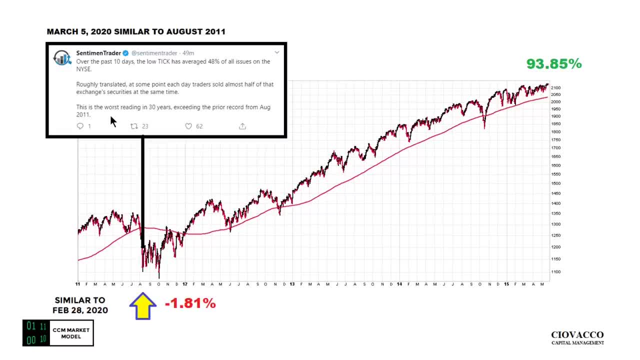 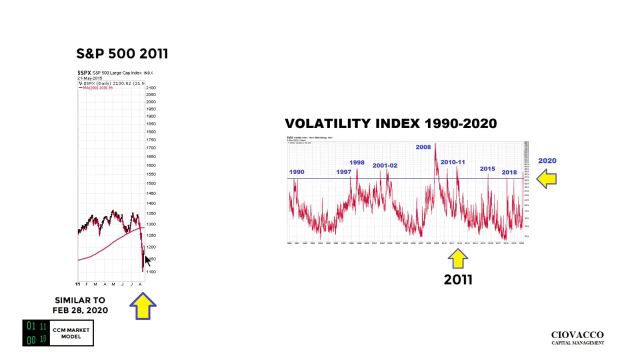 I see this is the worst reading in 30 years, exceeding the prior record from August of 2011.. August of 2011.. Something that just happened this week ties the present day to this period here, and something that just happened last week ties the present day to this period here. 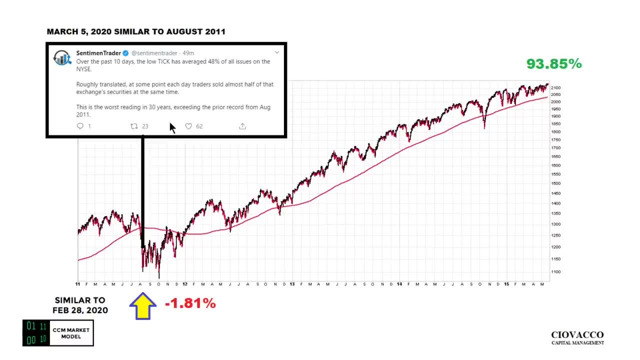 So this piece of new evidence aligns with the theory that the 2011,- 2011 case may be beneficial from a knowledge perspective walking forward, And this case here tells us that it could be very, very difficult and very, very volatile for several more weeks. 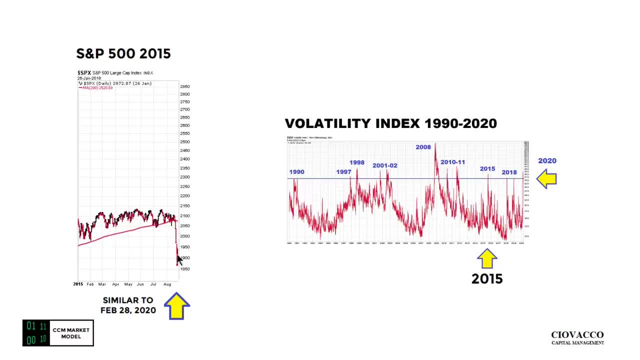 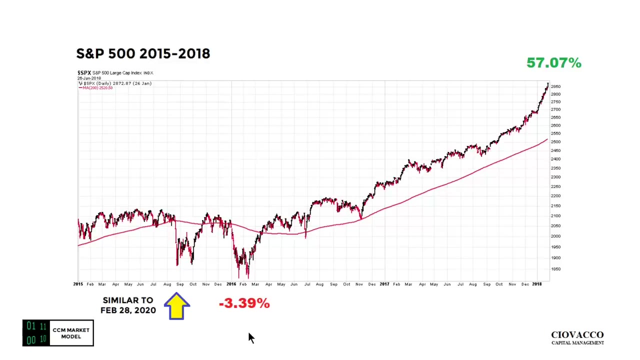 2015 case: an extremely scary and waterfall-type plunge here. Spike in volatility expectations in the VIX here very, very similar to 2020.. Walking forward from this point here, it helps us keep very realistic expectations about what the coming weeks and or months could look like. 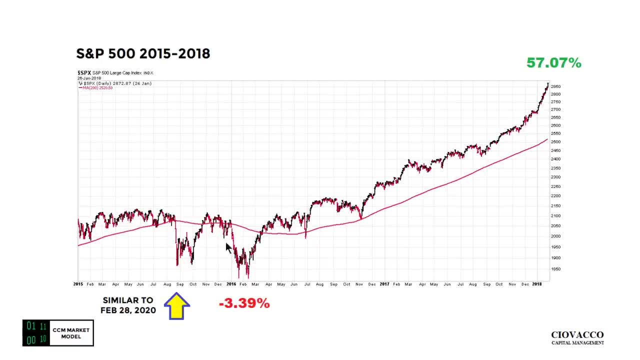 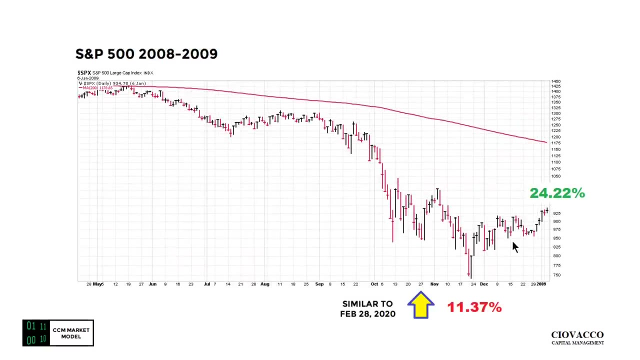 As we stated in last week's video, our goal in this area here, which is similar to the present day, is to get properly aligned with the resolution trend, Whatever happens after this. in this case, it was bullish In this case. 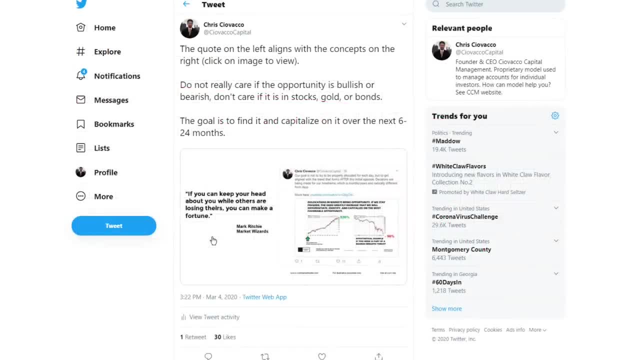 after this rally it was bearish, As noted on Twitter this week from the Market Wizards: if you can keep your head about you while others are losing theirs, you can make a fortune Walking forward. in the present day, we don't care if the opportunity is a bullish opportunity or bearish opportunity. 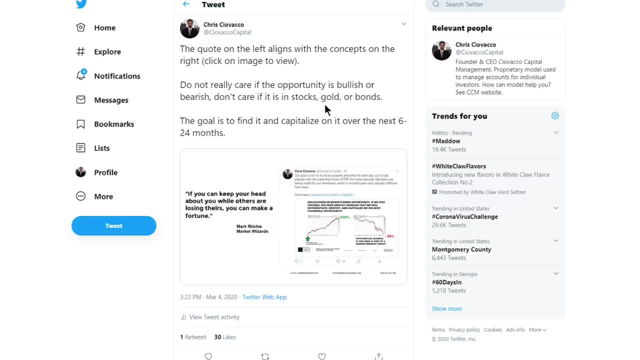 We don't care if the opportunity is in stocks, if it's in gold or if it's in bonds. The goal is to identify the opportunity and capitalize on it over the next six to 24 months And if you're a client. 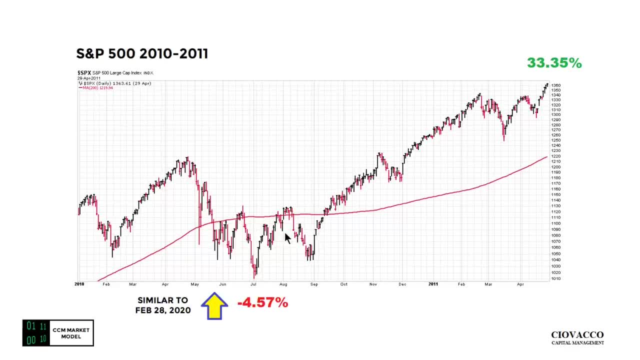 that means it may be messy for a while. Focusing on the short term in a case like this can be very, very, very damaging to your returns. Ask yourself here: do these day-to-day fluctuations really amount to much of anything? looking back, 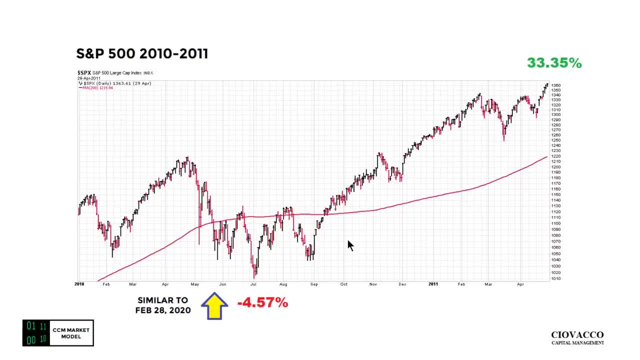 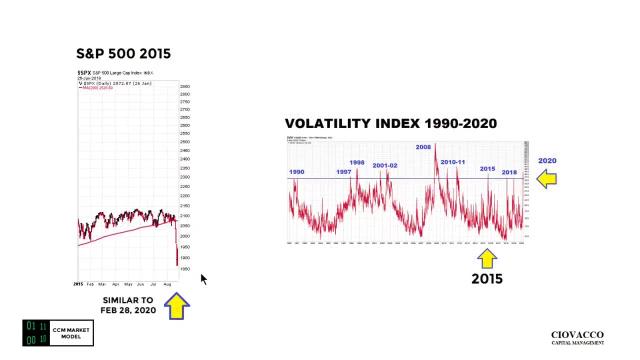 The answer is absolutely positively no, And, as we wrote on Short Takes on Monday of this week, it's 100% normal and to be expected for a market to look extremely irrational after a plunge like this. What happened in this case if we were able to remain rational while the market was? 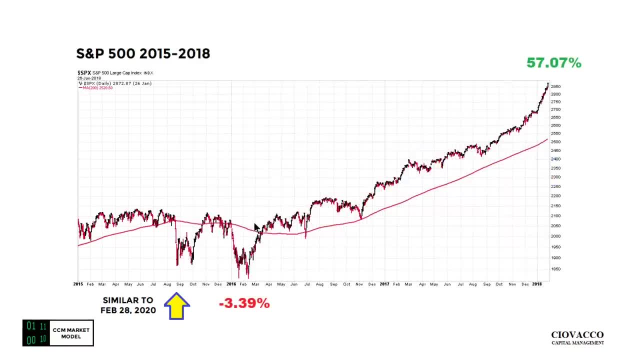 for the most part, appearing to be irrational If we maintained our focus in here. additional drawdown of 3.39% from this low here- That sounds awful at this point And it would be extremely painful at this point. That's a big number. 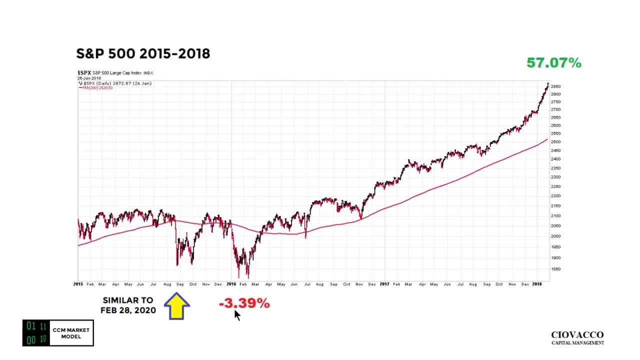 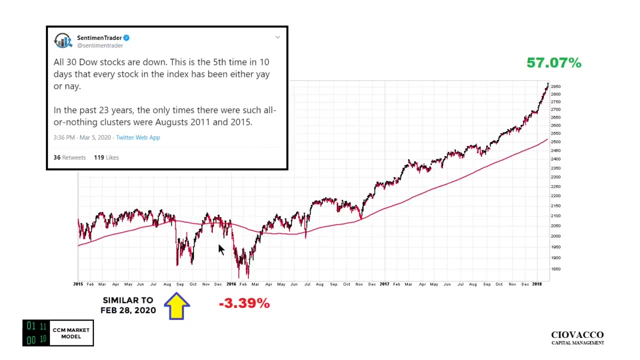 But this number here takes on a whole new meaning in this context, here in the upper right hand corner of your screen. Once again, we started this study earlier in the week. Sentiment Trader on Thursday: another piece of data that ties this period to the present day. 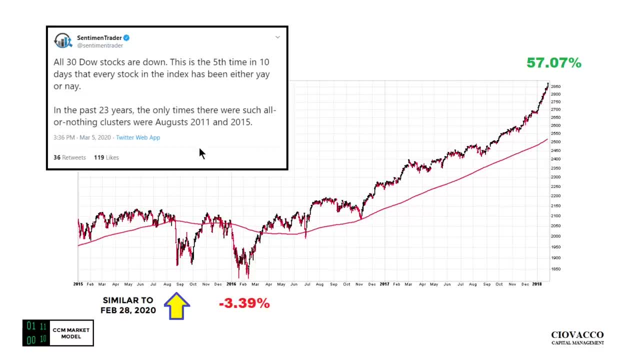 All 30 Dow stocks were down on Thursday. This is the fifth time in 10 days where either they were all up or they were all down In the past 23 years, the only times there were such all or nothing clusters. 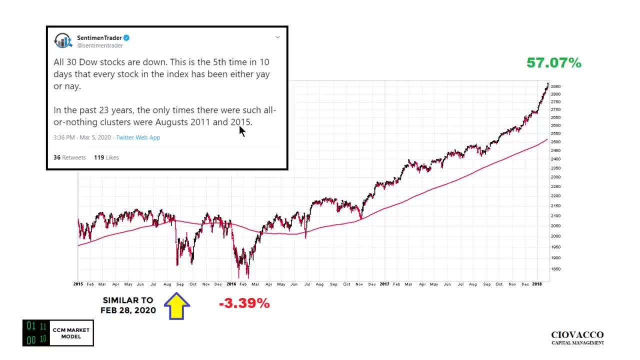 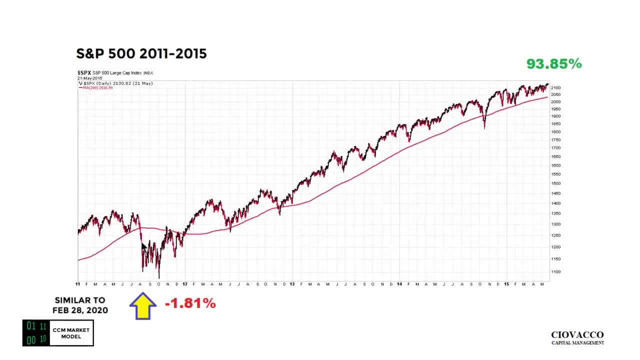 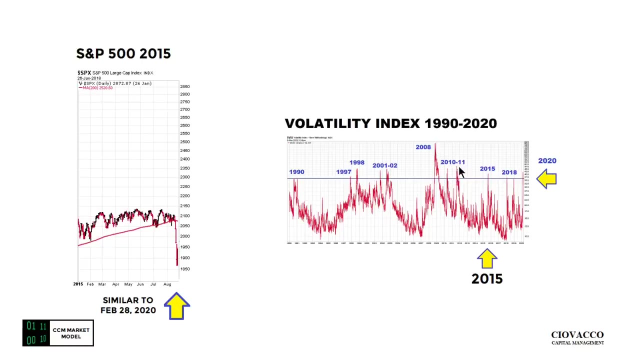 August of 2011 and 2015.. In our study, 2015 and in our study, August of 2011.. In our study, a big spike in the VIX 2015,. a big spike in the VIX in 2011.. 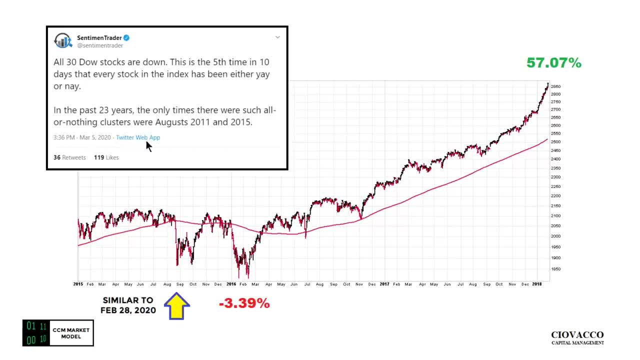 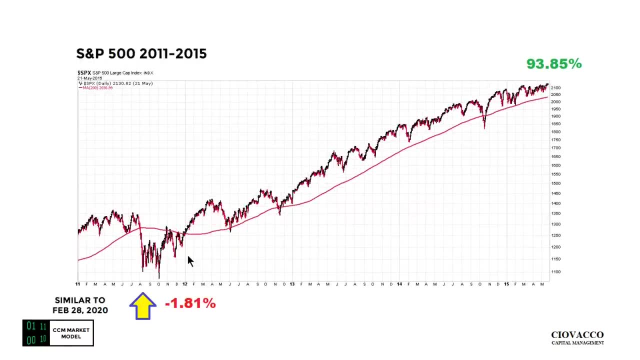 A piece of data from Thursday March 5th aligns with, rather than contradicts, this study here. And it aligns with, rather than contradicting, this study here. None of it predicts the future. It simply speaks to the probability of good things happening. 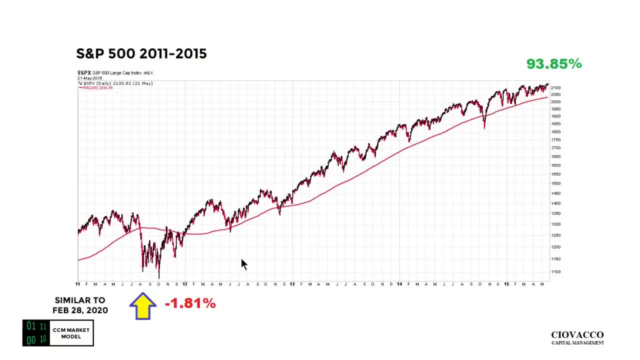 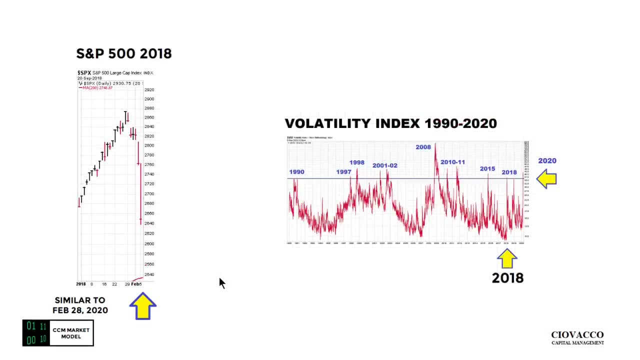 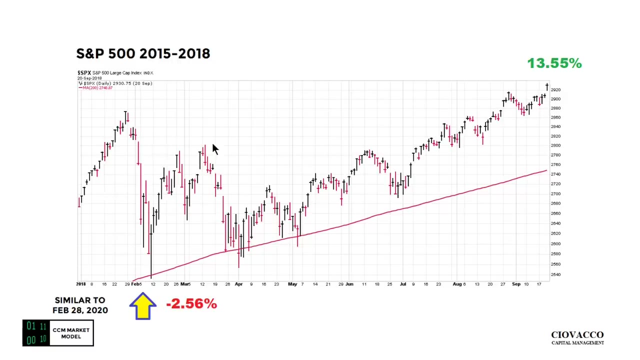 relative to the probability of bad things happening walking forward. The probability of bad things happening is never zero. 2018 case: big, scary plunge, big spike in the VIX walking forward. If you were able to maintain your composure in this area here. 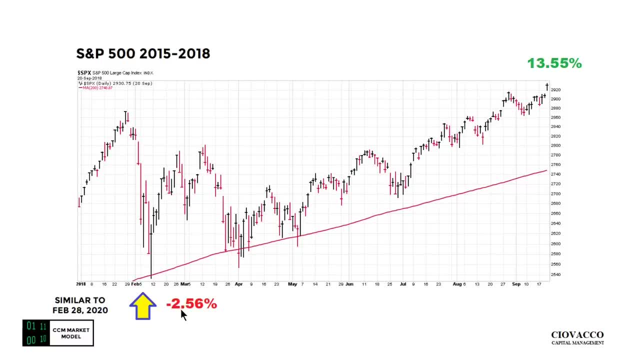 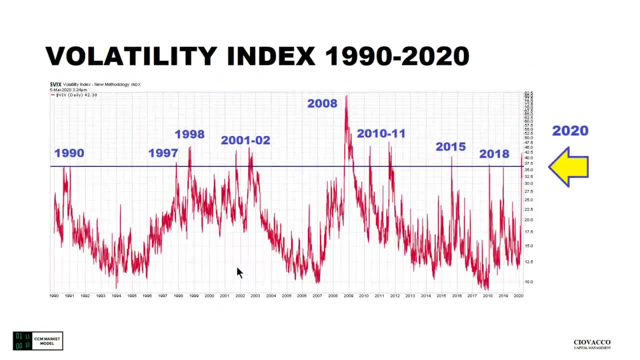 eventually, the market righted itself after an additional drawdown of less than 3% and it tacked on 13.55%. Before we look at a summary of the results, it's important to note we have included every single case, using all the data that we have. 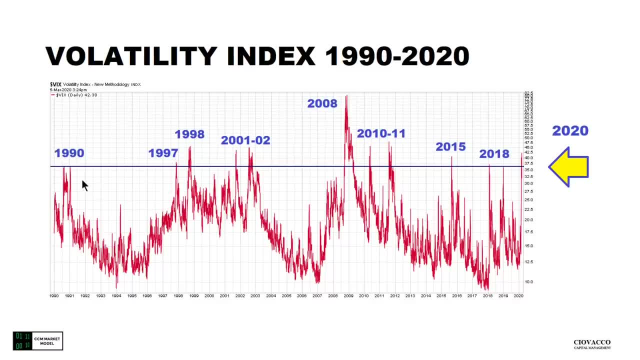 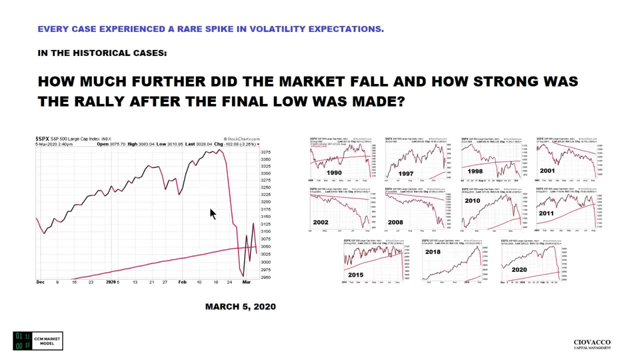 and we have included bear market cases and bull market cases. These are the only cases that are similar to what just happened Only 10 previous times, dating back to 1990.. Let's double back to our original question: How much further did the market fall in each case? 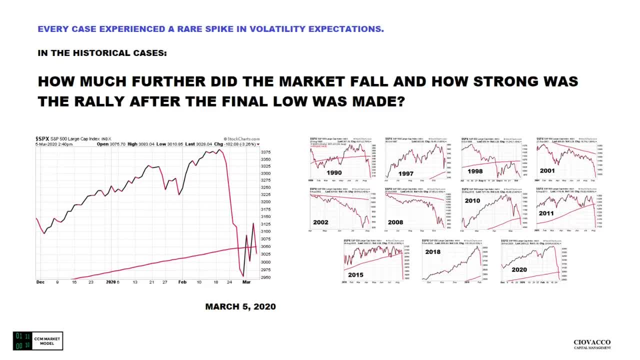 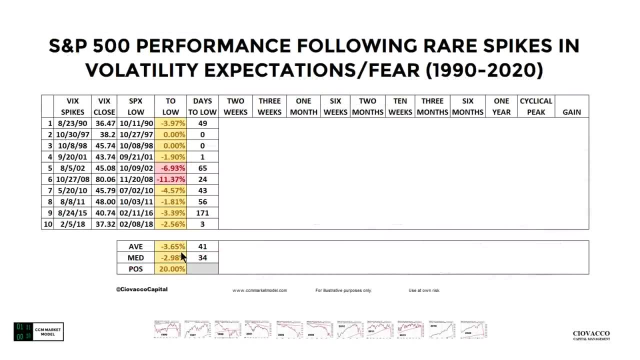 And how strong was the rally after the final low was made? If we put all 10 cases into a table, the average additional drawdown from the day that's similar to the close on Friday, February 28th 2020,. 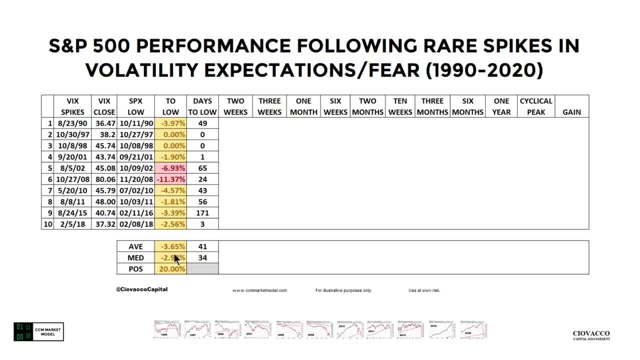 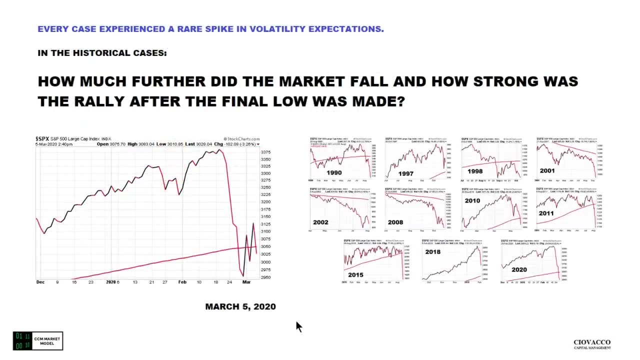 as of this recording was 3.65%. The median drawdown roughly 3%. In two of the cases there was no additional drawdown. These are the same figures that we just covered in the charts, and history tells us that if we're able to maintain our composure in here, 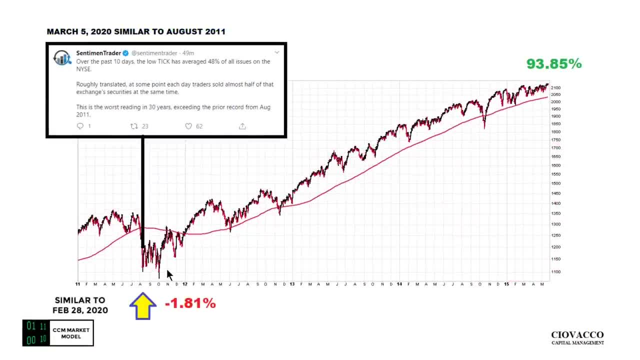 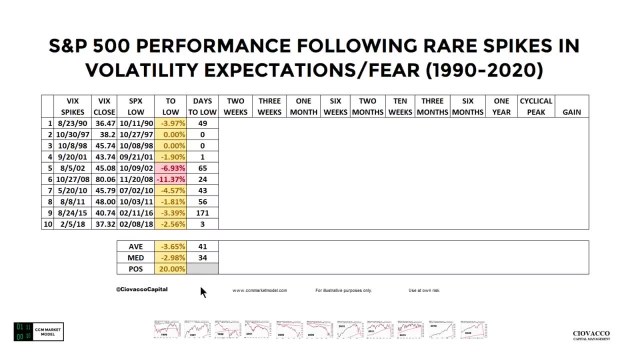 and if we're able to maintain our composure in what could be a very, very difficult few weeks or few months, but will feel like excruciating pain walking forward in the form of roughly a 3% additional drawdown from the low that we've already made. 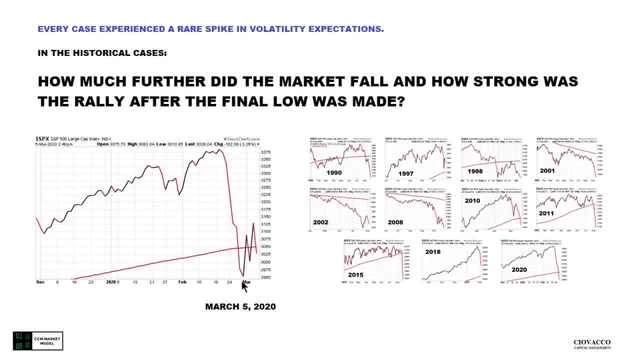 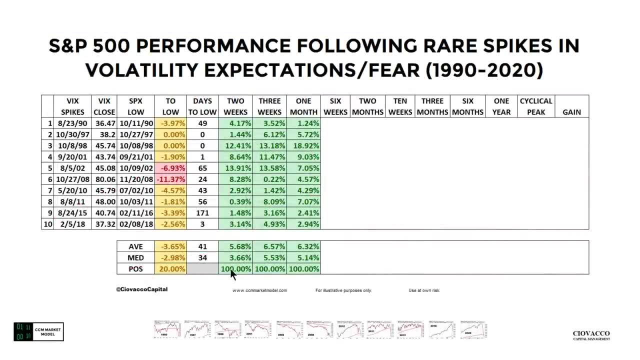 could feel a lot better in a few weeks. Two weeks out in the historical cases, walking forward to the point that's similar to February 28th, 100% of the cases were higher. Three weeks out: 100% of the cases were higher. 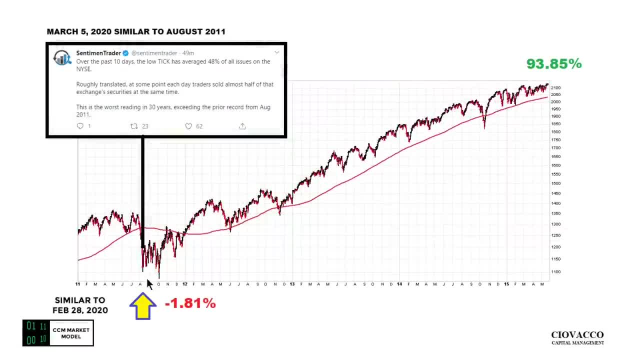 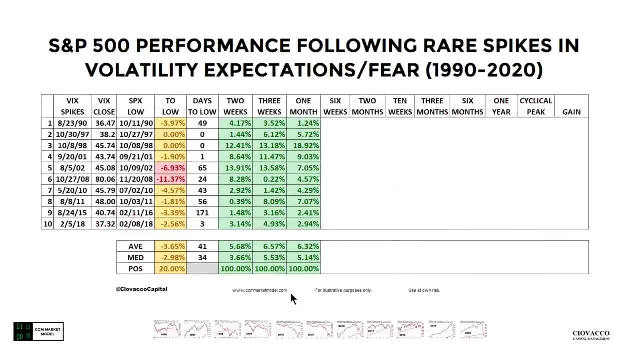 One month out, 100% of the cases were higher. Anecdotally, that's this type of move in here off the oversold low. Then after the first few weeks, typically there's some give back in here. 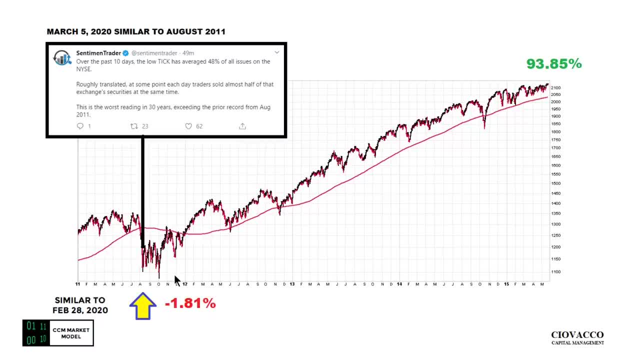 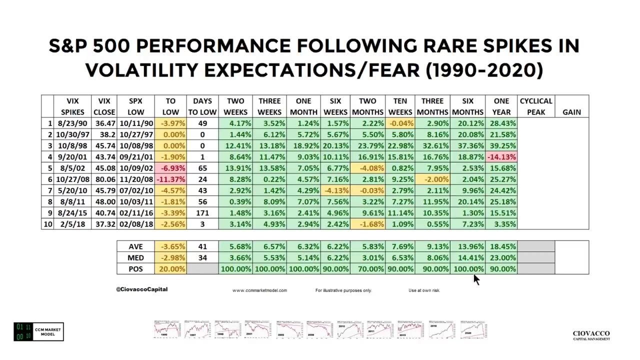 This area here speaks to having realistic expectations about the market making a lower low, even if really good things are to happen walking forward, In the historical cases things tended to be quite a bit more calm six months out, 100% of the cases were higher. 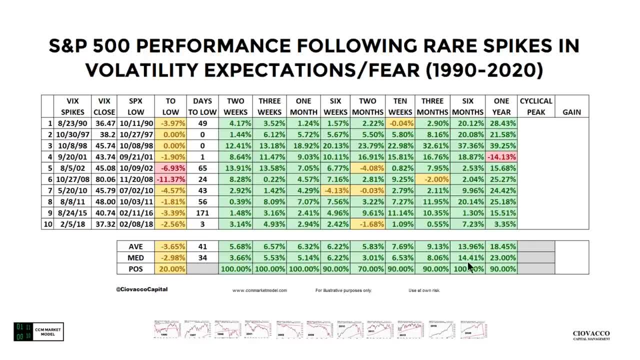 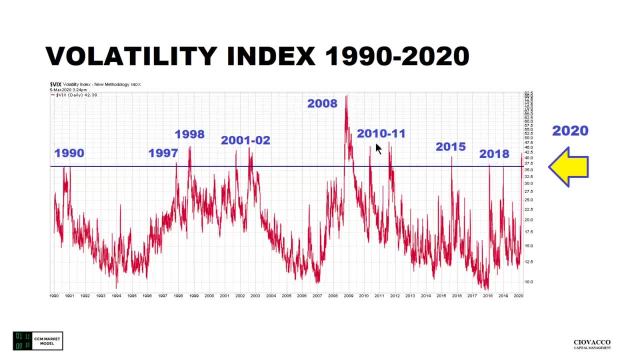 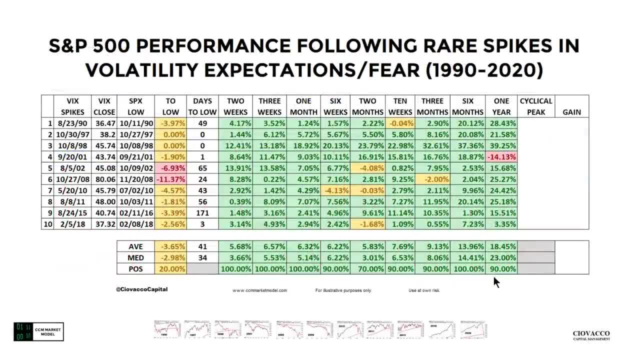 or a peak that's coming relatively soon. In 90% of the cases, the stock market was higher a year later. Average gain 18.45%, The median gain 23% And maybe more importantly, for investors it's very. 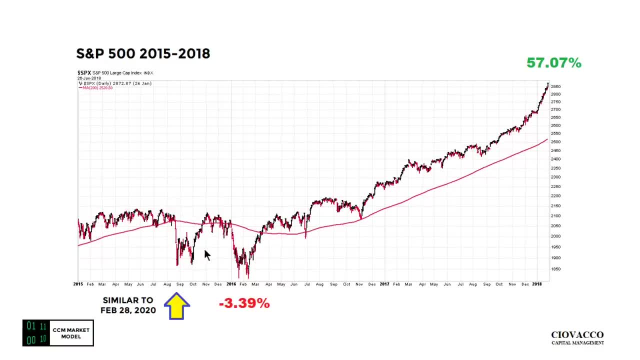 very easy to shrink down your time horizon when things get volatile And if we lose our focus in here turn out to be very, very costly from a longer term perspective. In this case, the gain from the final low to what we'll call the cyclical peak. 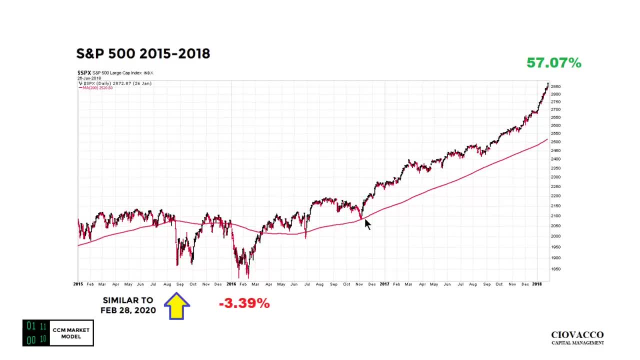 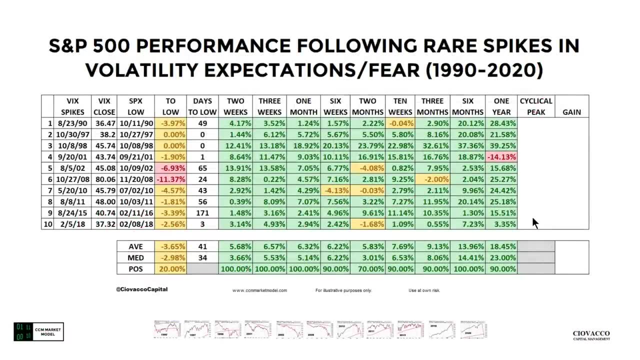 which can be months out, years out, days out or even just weeks out. In this case it was 57%. What does that number look like For all of the cases if you navigated properly during the very, very difficult bouts of volatility? 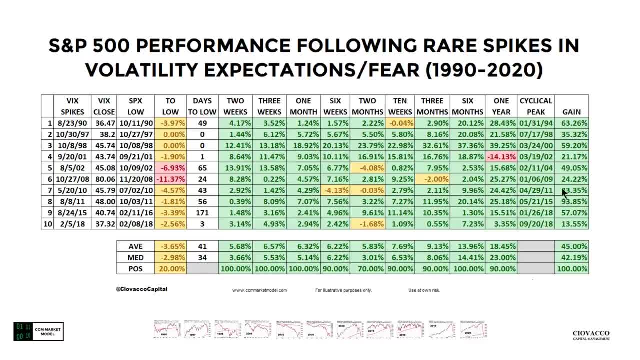 in every single case. after the market found a bottom, really good things happened. This is your average pain right here. all of the cases. This was your average gain: 45%. the median 42%. Every single case: patients was eventually. 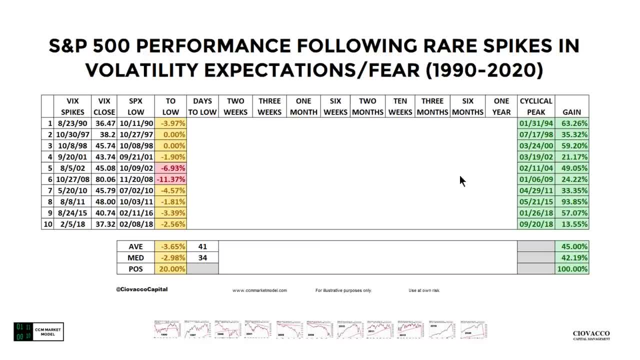 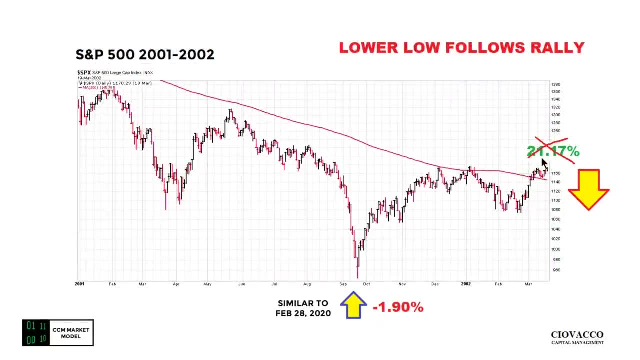 rewarded. Even these numbers here eventually turned into really good numbers here We want to make it abundantly clear: This case and this case occurred within the context of a bear market. Yes, we did get a very, very nice 21% rally from this oversold condition here. 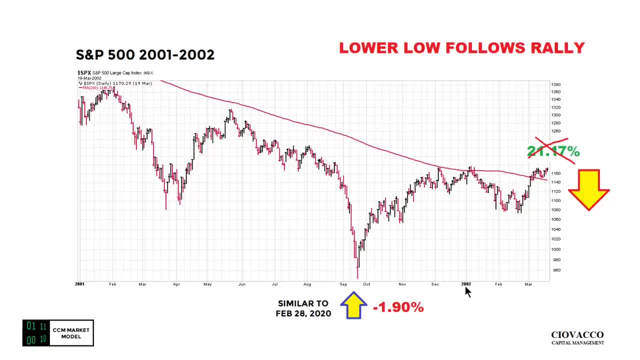 The market doesn't bottom until October of 2002.. How is this helpful? It's helpful because patients from the oversold condition and after the big spike in volatility expectations was rewarded for several months and in a big way. That is helpful walking forward in the present day. 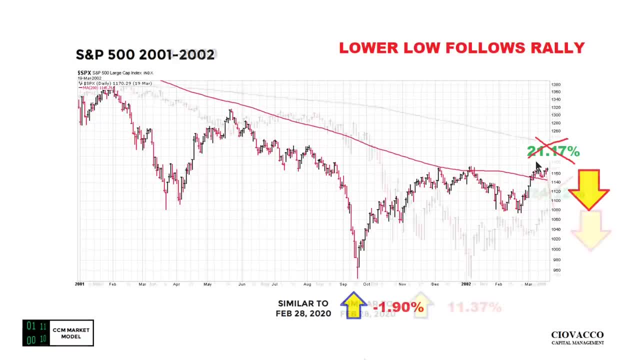 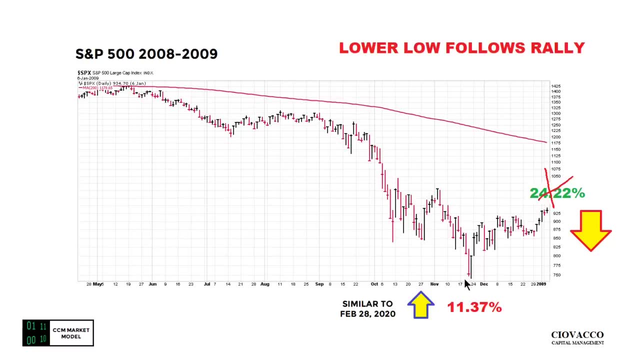 Even in a horrible case, good things happened in the short term. Even in a horrible case, good things happened in the short term. from the extremely oversold condition, This gain here was totally wiped out, Something that we have to be aware of. 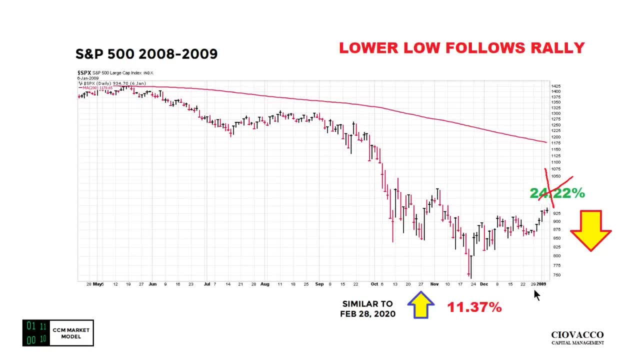 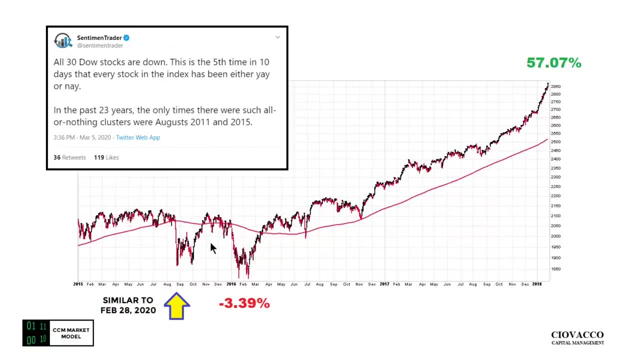 the market did not make the final low until March of 2009.. It's very, very easy, when something like this is going on in the stock market, to just say: I've had enough In every single case if an investor kept their eye on the ball. 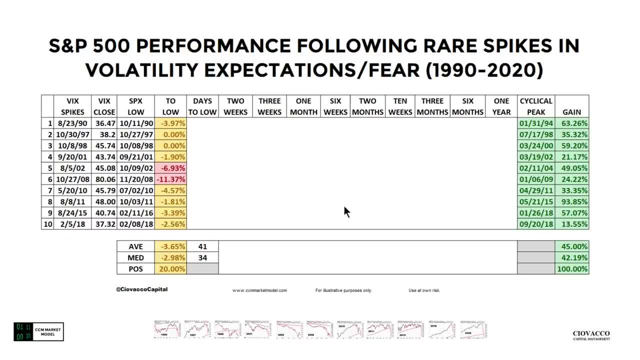 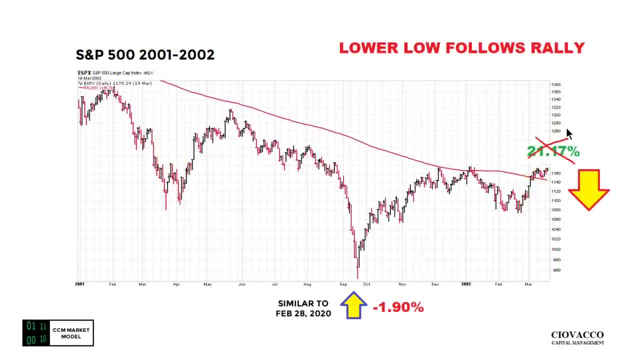 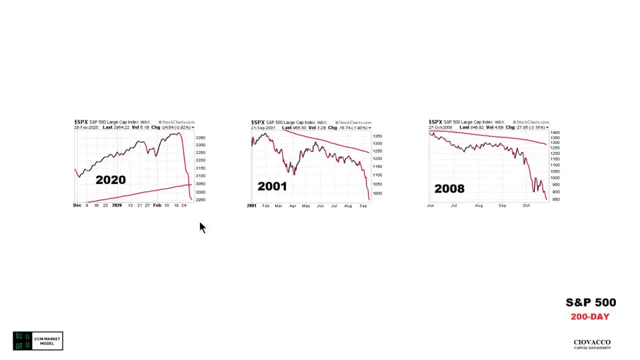 and, more importantly, on their timeframe, which should be longer term. really good things eventually happened And, yes, some bad things happened along the way, But it's also noteworthy These cases here on the day of the volatility spike that's similar to February of 2020,. 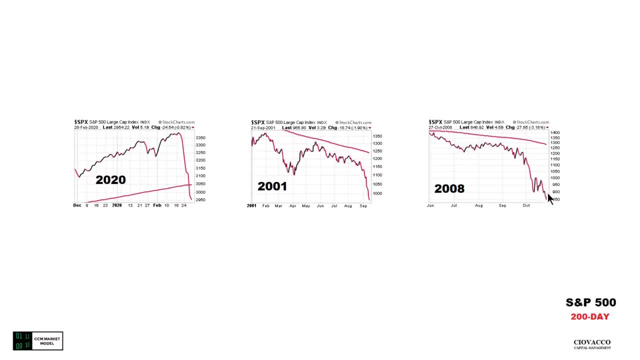 the day of the volatility spike. that's similar to February of 2020, the market's profile really doesn't look anything like the present day. Price is below a downward sloping 200-day when that happens. in this case, Price has been down below a downward sloping 200-day for several months in 2008.. 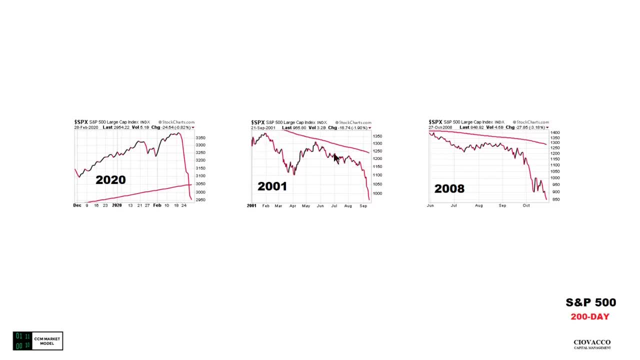 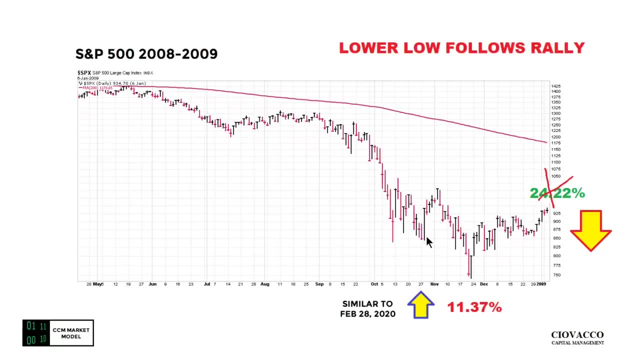 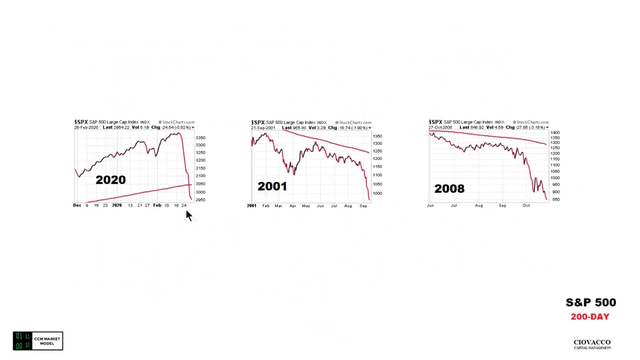 This is a clear and existing downtrend- a clear and existing downtrend. not the case here. And it's not surprising that a clear and existing downtrend had a sharp counter trend rally and was followed by lower lows. The mathematical profile of the market here is infinitely better than the market here and the market here. 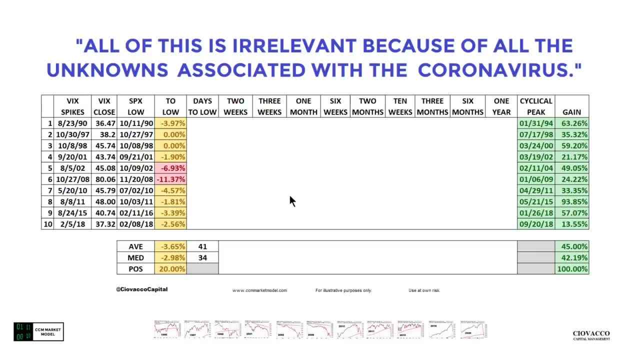 which simply speaks to probabilities walking forward. If you're relatively new to the stock market, you might be saying all of this is irrelevant because of all of the unknowns associated with the coronavirus. Common sense tells us that when we see a plunge like this, 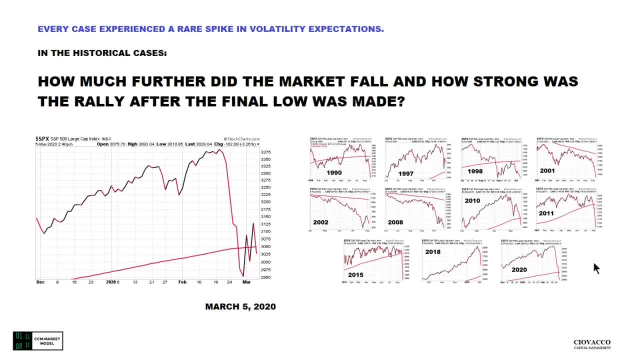 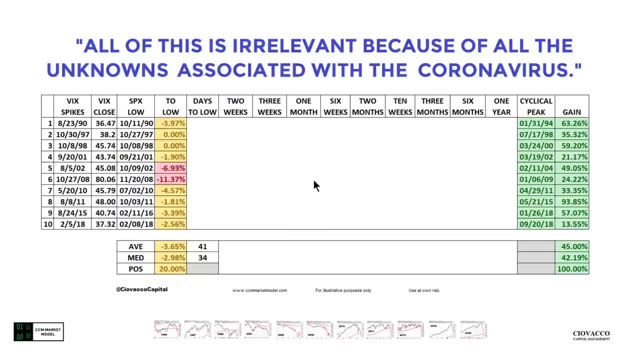 very concerned about, Just as you could say rationally and logically in the present day that all of this is irrelevant because of the unknowns associated with the coronavirus. In each case, we could have inserted something here. 1990, we had a savings and loan crisis in the rearview mirror and Iraq invaded Kuwait. 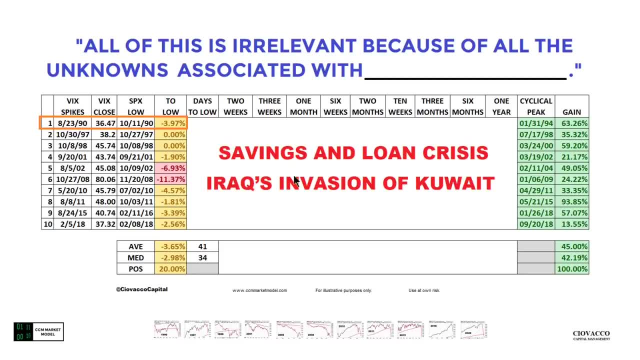 disrupting the oil markets. Lot of unknowns in here 1997 case. big spike in volatility expectations Happened for a reason: Had a very, very serious Asian economic crisis and a major securities firm collapsed in Japan. You've heard about Lehman Brothers in the United States. 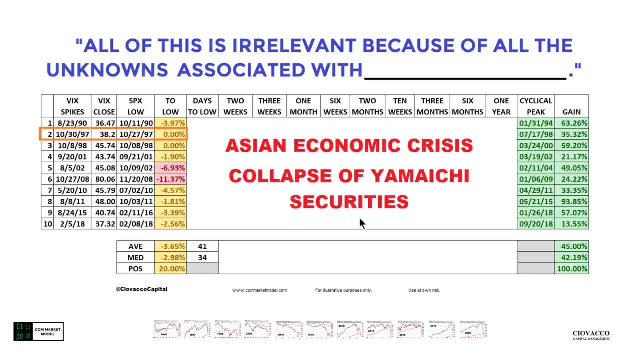 That has a tendency to get people a little bit unnerved. Serious situation in 1998, with a Russian debt default and a crisis, Lot of unknowns associated with the bursting of the dot-com bubble. All of this is irrelevant. relevant because of all the unknowns associated with the failure of Lehman Brothers. You really 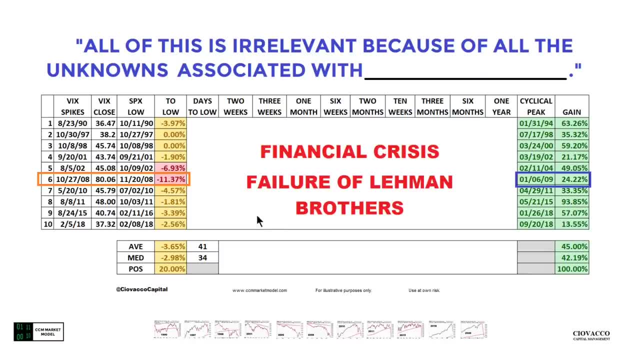 can plug something in in each case, And in each case it sounded very, very logical. 2010, we had the flash crash. The markets are unstable. Anything can happen. walking forward, We have unknowns and uncertainty that we've never seen before. 2011, European debt crisis. This is 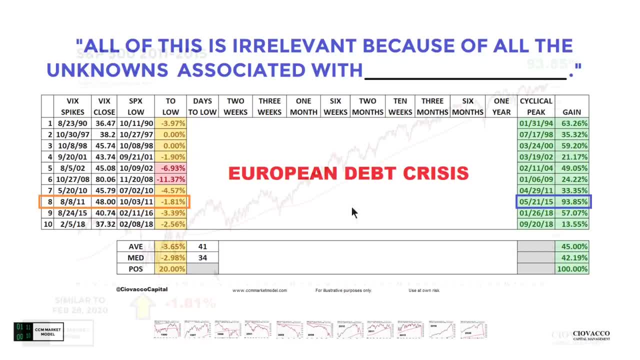 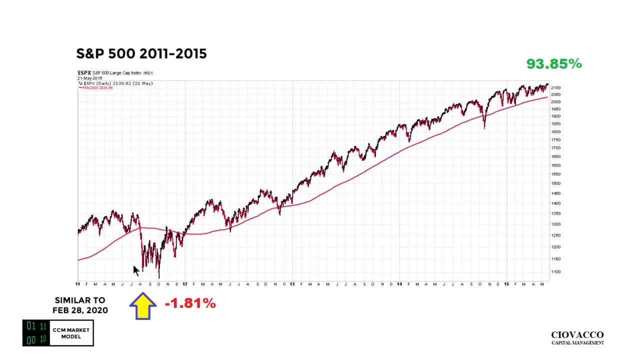 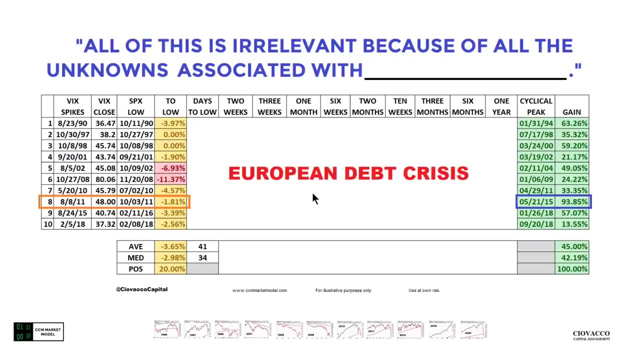 a very, very, very serious situation, And when we have very, very serious situations, we can get market dislocations and a ton of wild swings. Sound familiar? If you don't know about the European debt crisis, go read about it. It was very, very serious. You know what happened walking forward. 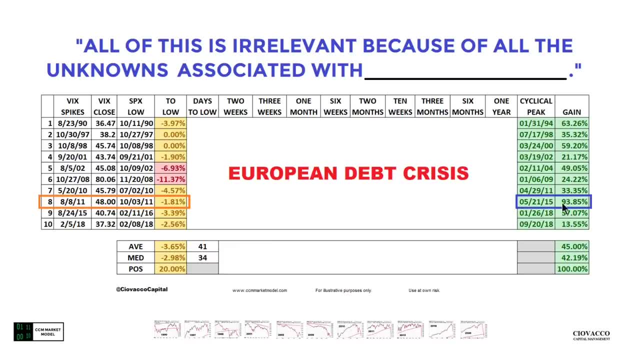 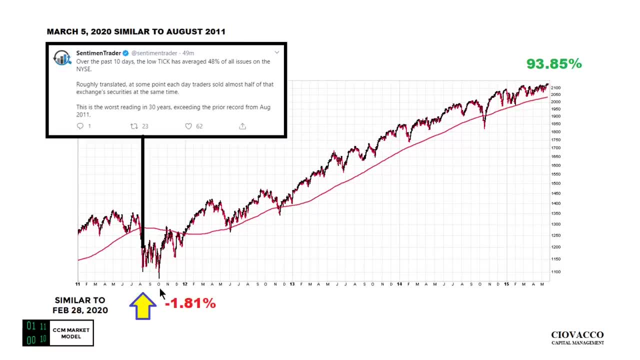 to the next big peak, A 93% gain. But it was not easy to get from point A to point B And we would not expect it to be easy walking forward in the coming days, in weeks and possibly even months. We 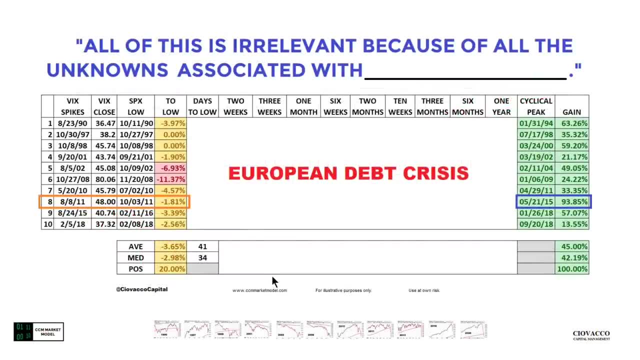 have to have very realistic expectations. Well, 2015 must have been a cakewalk. It was not a cakewalk. Big, big concerns about global recessions and negative interest rates, in the upcoming Brexit referendum and the upcoming US presidential election. From this crisis point, 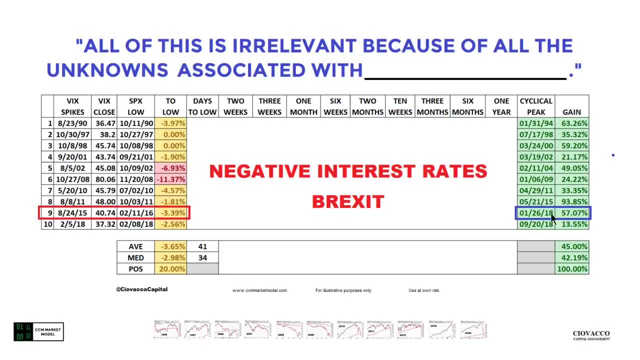 here, which is similar to the present day. in this point here, 57% gain between point A and point B. Between point A and point B, the futures- S&P 500 futures- went limit down twice. There was a lot to be concerned about And if you're in the business, 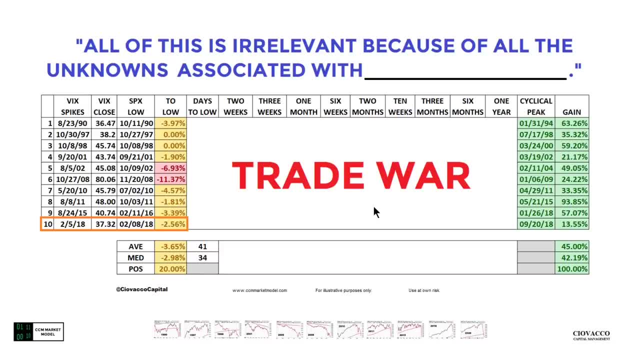 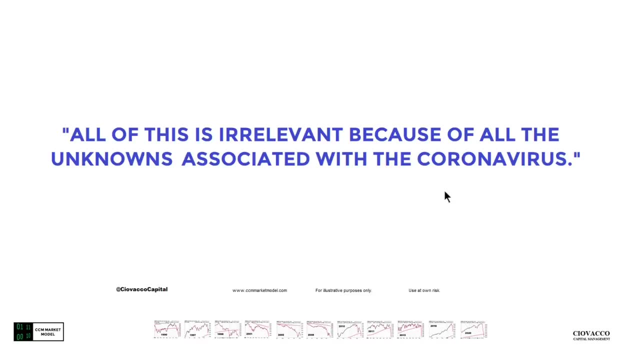 you probably heard this more than once over the past 14 months: All of the charts, all of the data in this analysis. it's irrelevant because of all the unknowns associated with the trade war. You still might be saying: none of that compares with the coronavirus. 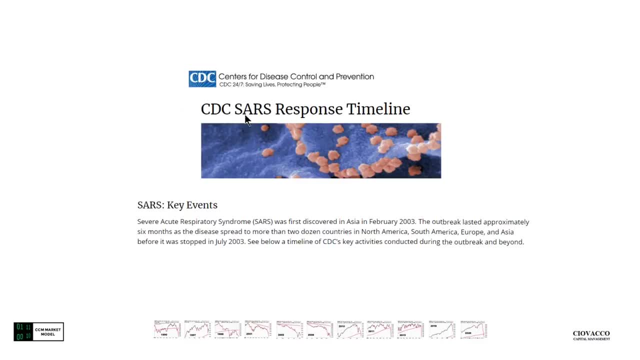 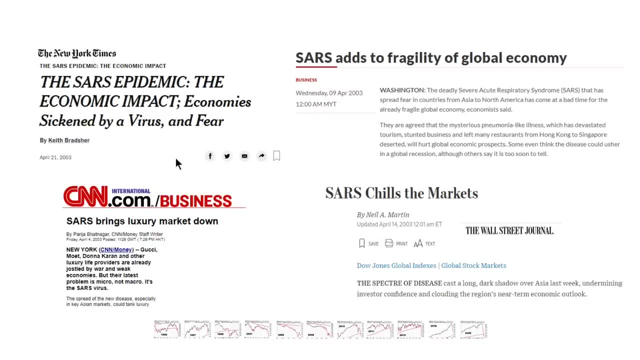 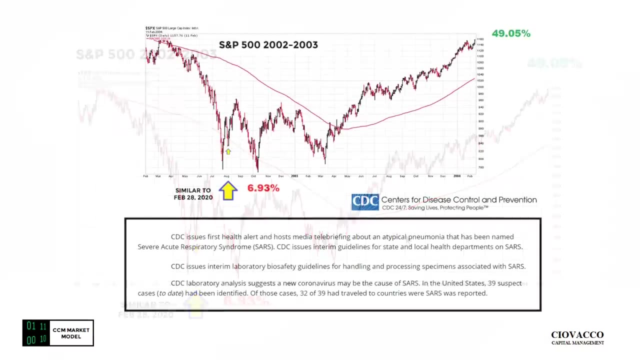 I've been around a long time. I remember hearing something very, very similar to that when SARS was around. These are all headlines from 2003.. Very, very similar headlines to what we've been seeing in recent weeks. Just so happens that 2003 was included in our study. 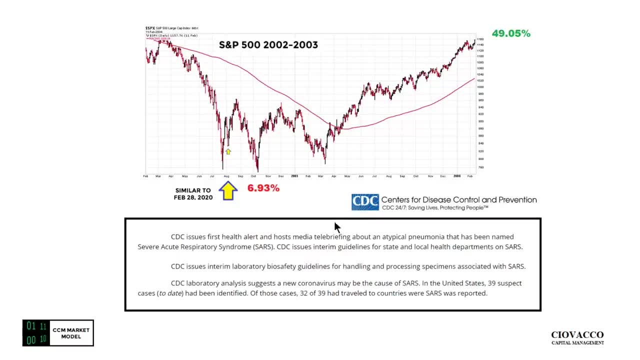 and this is the timeline for SARS right off the CDC website. So it might be helpful to know: Is this timeline over here about SARS? No, it is not. This is 2003,. March 15th, March 22nd, March 24th. 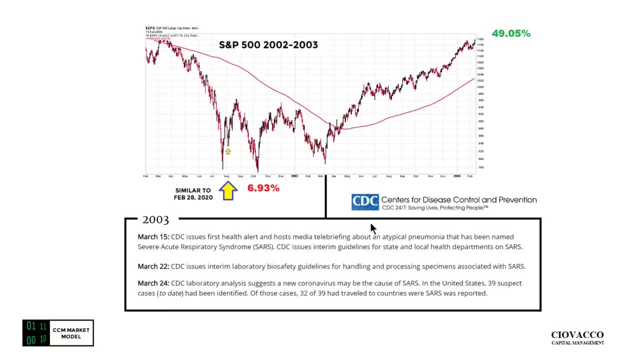 and there are a ton of dates listed on the website in March. walking forward, Here's March on the chart of the S&P 500, 2003.. These were the headlines that we were dealing with and this is what happened in the S&P 500.. 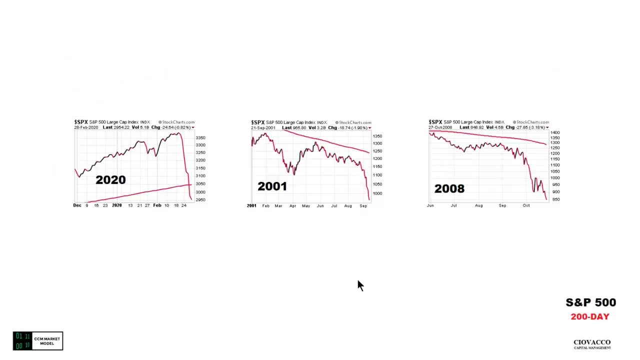 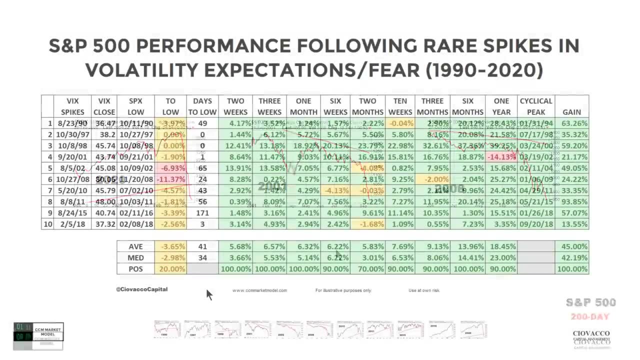 Is it possible in the present day that we are already in the early stages of a bear market? Absolutely positively, yes. As we have stated over and over and, over and over again in these videos, we do not, never have and never will make any decisions based on a historical study. 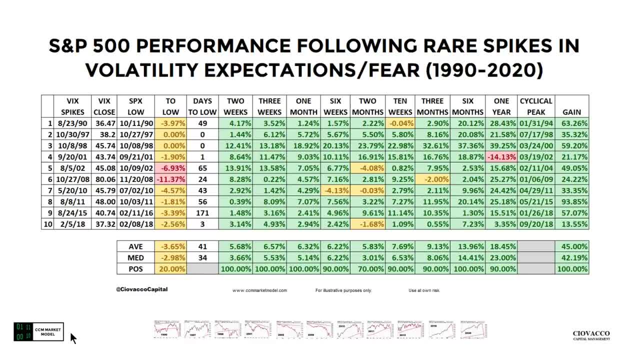 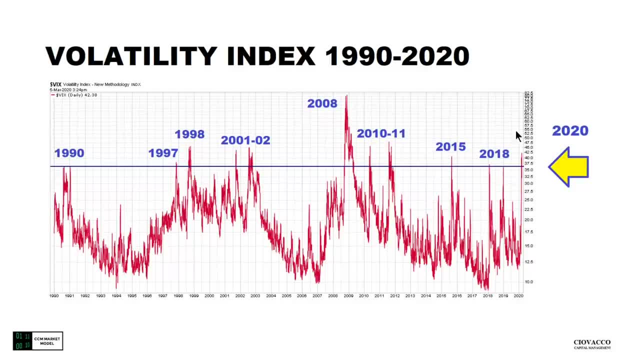 100% of our decisions are based on the facts in front of us today and the data tracked by us. This is the data in the present day. It's really impossible to understand what this may mean in the present day if we don't perform this type of analysis in a detailed manner. 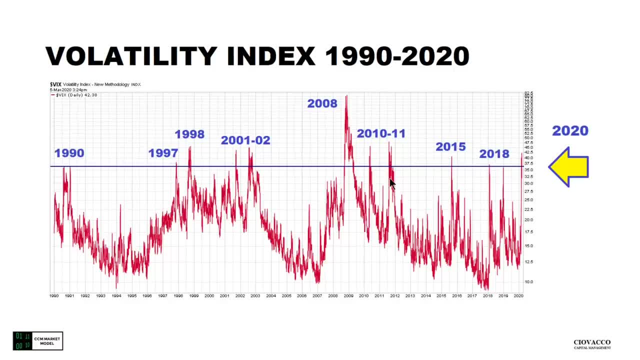 and it cannot be done by just looking at the chart. If you didn't have a reference point and somebody told you it was 98 degrees outside, and you had no experience or no historical data, 98 degrees would mean absolutely nothing to you. This is the data that's in the model. 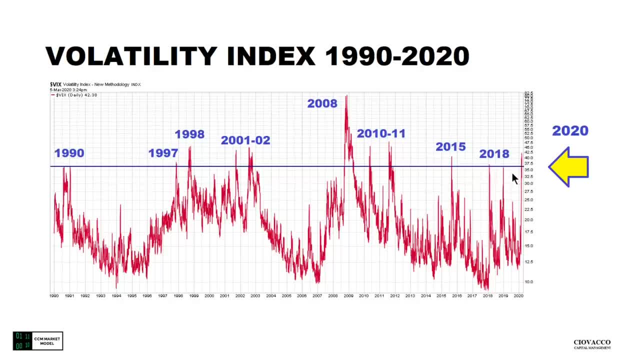 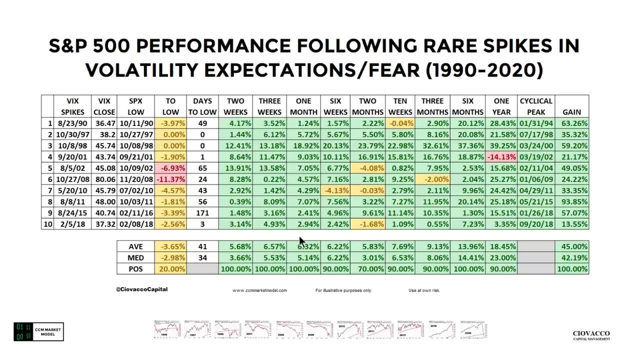 This helps us understand the present day data in a historical context. In the historical cases, this is what happened next: Simply context, not a forecast. And what we're about to cover is simply context. It has nothing to do with making decisions walking forward. 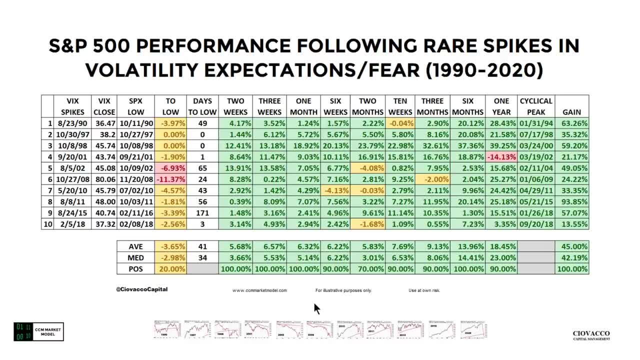 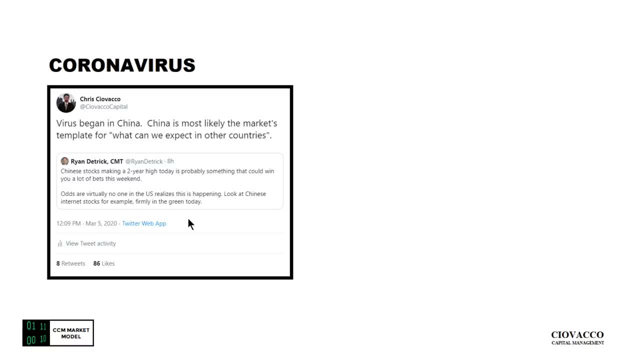 However, from an execution standpoint, it might be helpful to know how is something like this even remotely possible in the present day, given we're dealing with the coronavirus? There are many possible answers to that question, but let's throw out one to provide some context. 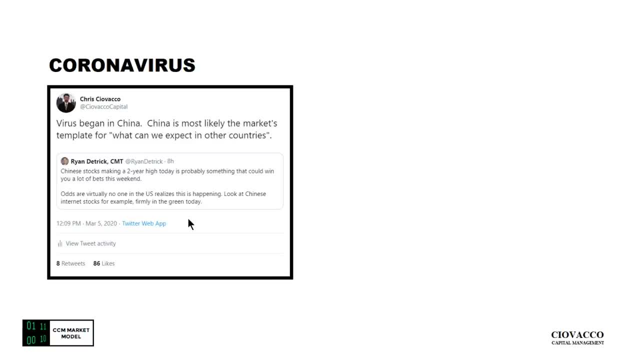 Once again, this analysis has nothing to do with how we're allocated today and how we will allocate going forward. The virus originally had a major impact in China, And now the virus is spreading to other countries, which is pretty much inevitable. It's pretty much inevitable that the number of cases in the United States 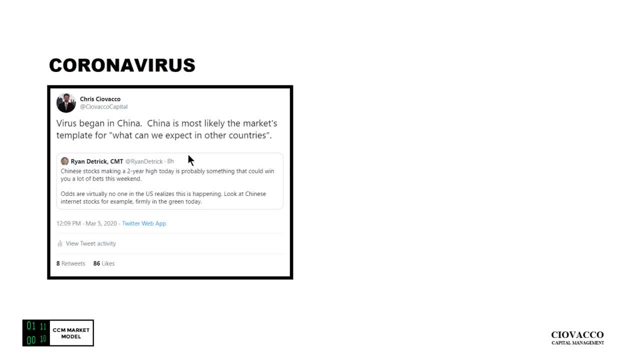 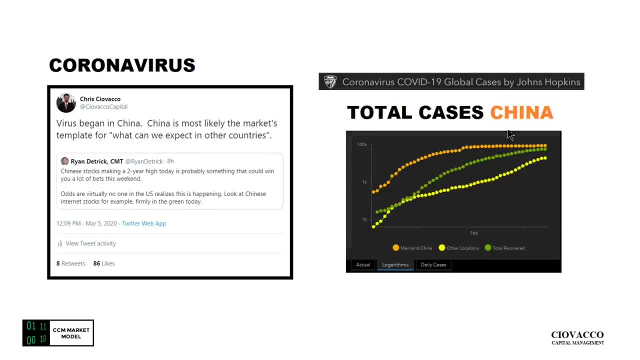 are going to increase significantly. It is quite possible that the market is saying China is the template for other countries walking forward. There's a John Hopkins chart here: Total cases in China in orange. This is February here. Notice the look of the chart here. 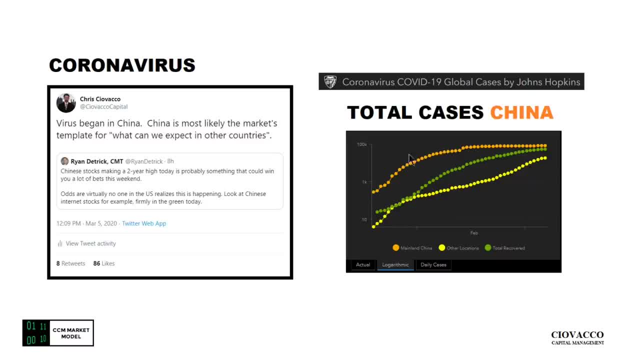 So this would be A realistic, a reasonable expectation for the United States walking forward, potentially A big spike in some shape form or fashion in terms of the shape of the curve. It's also possible that a few weeks down the road, 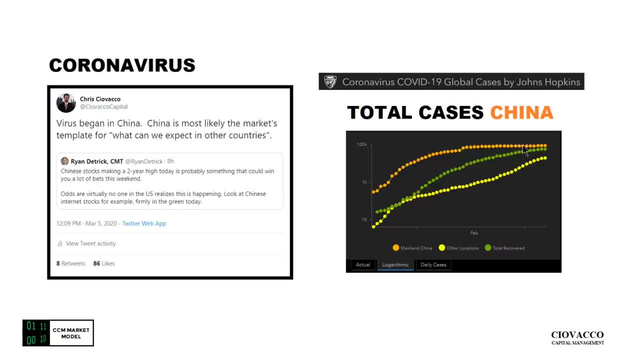 this is a reasonable expectation for the curve of cases in the United States. Hypothetically, if that's the case, if every single country develops a curve like this and China's curve stays like this, then it is possible that the market will say: 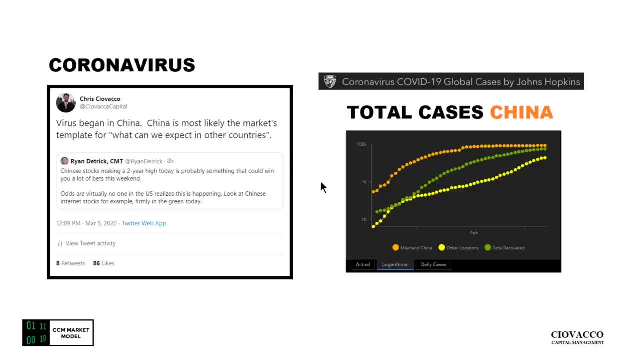 this is not going to cause a global depression. Conversely, if this line turns back up, it's very, very difficult to believe that that would be good for the financial markets. And yes, there are differences between China and the other countries, But there are also a lot of similarities. 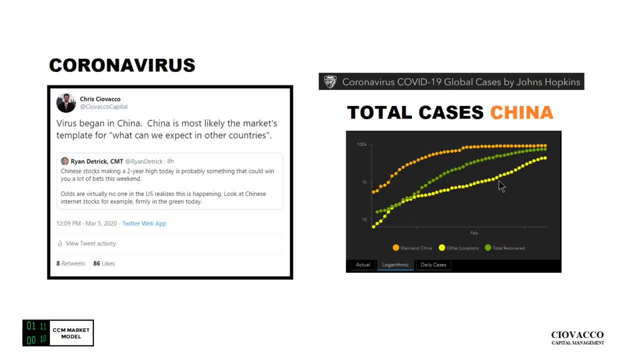 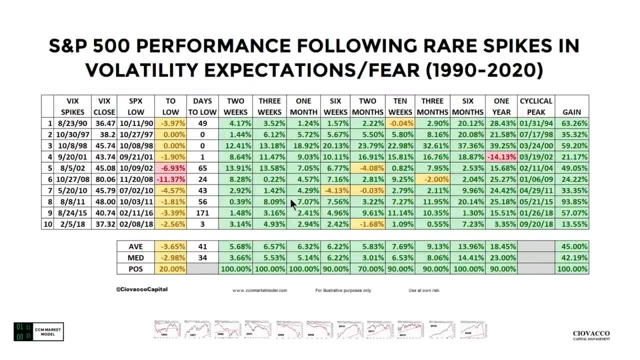 We're talking about human beings and the spread of a virus. If every curve develops like this, it's very, very easy to understand how something like this could happen from an extremely rare and oversold and lopsided condition. Here's an article dated February 12th: 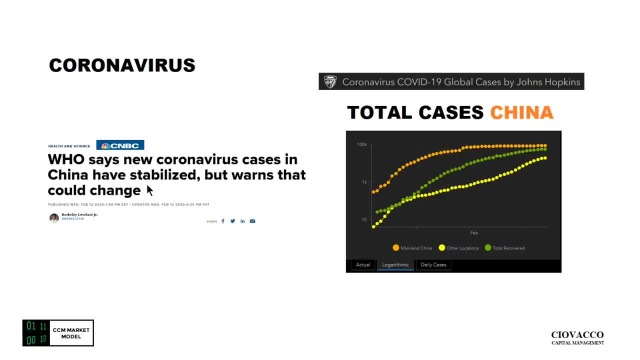 World Health Organization says new coronavirus cases in China have stabilized. This was written in mid-February about right here Seems to be pretty accurate. Seems that the new cases in China for now have stabilized. And if, for some reason, you don't agree with any of this, 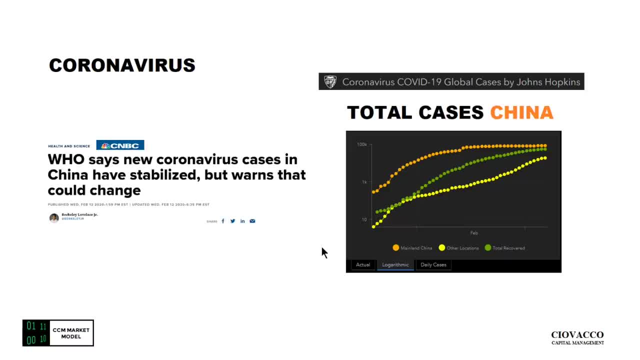 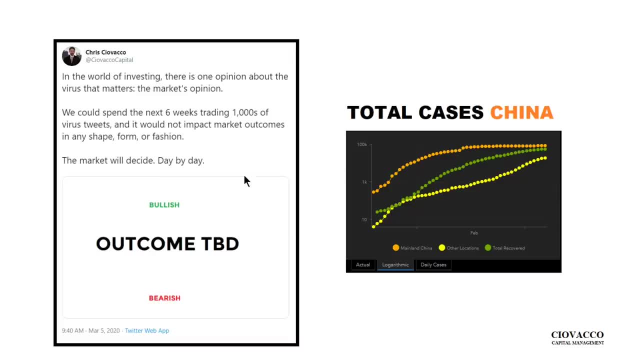 it really doesn't matter And it's really not worth debating. We don't make any decisions based on this. We make decisions based on the data, And that's relevant because in the world of investing, there's only one opinion about the virus. that matters. 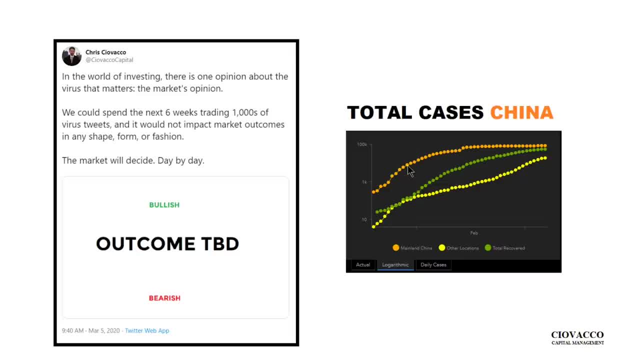 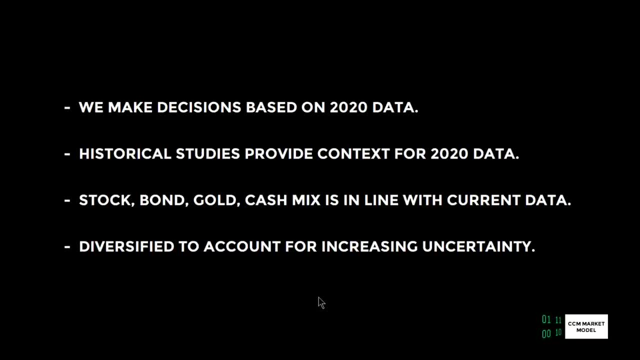 the market's opinion And we will continue to track the market's opinion via the hard data. In summary, we always have and always will make decisions based on the data that we have in front of us in the present day. Historical studies simply provide context. 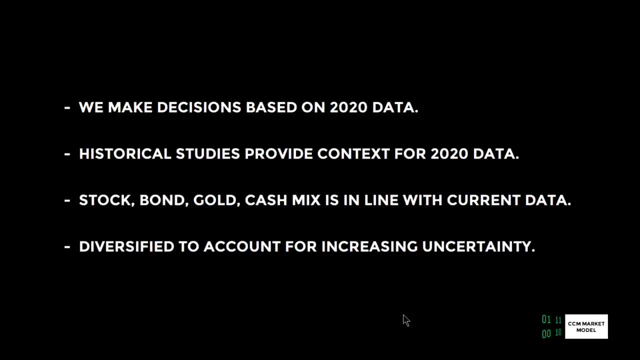 What does 98 degrees mean? What does 22 degrees mean For clients? our mix of stocks- bonds, gold and cash- is in line with the current data. If the data shifts in a material manner, we will make the necessary adjustments. 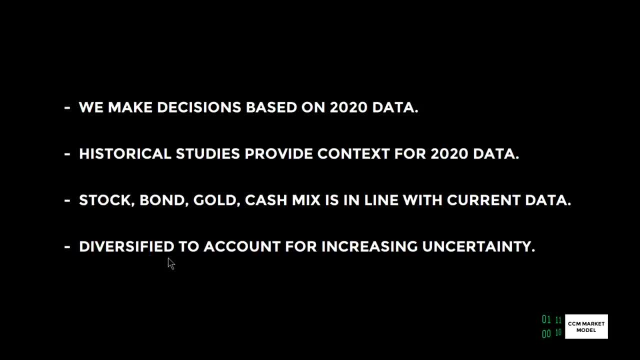 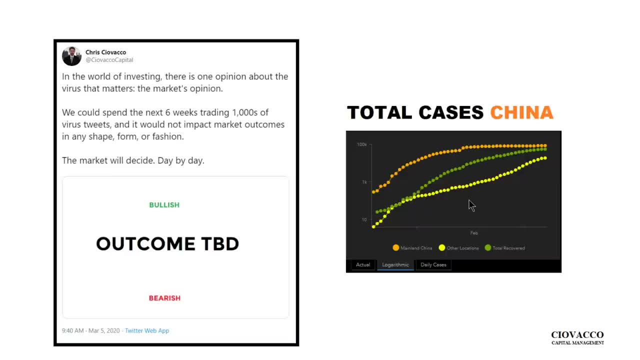 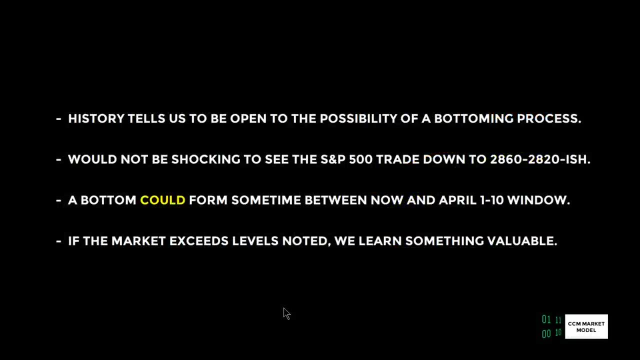 Notice. we are well diversified to account for the increasing uncertainty in the present day related to the virus, And that includes uncertainty related to all of this data. This curve could level out or it could start to rise again. History tells us to be open to the possibility of a bottoming process. 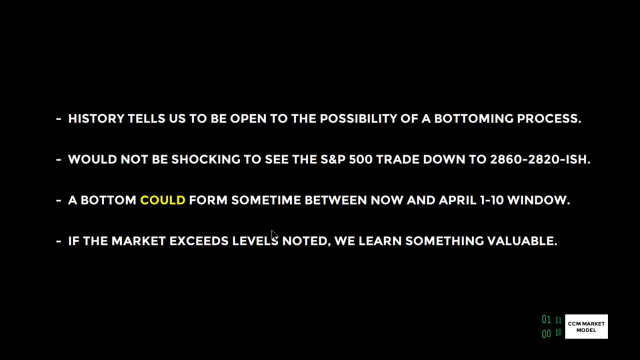 There is no question. price action between Monday and Thursday is following the script that we outlined on Short Takes Monday morning before the market opened. Will that continue? We have absolutely positively no idea. We take it day by day. Based on the study that we just covered, it would not be shocking to see the S&P 500 trade down to the 2860-ish to 2820-ish range. 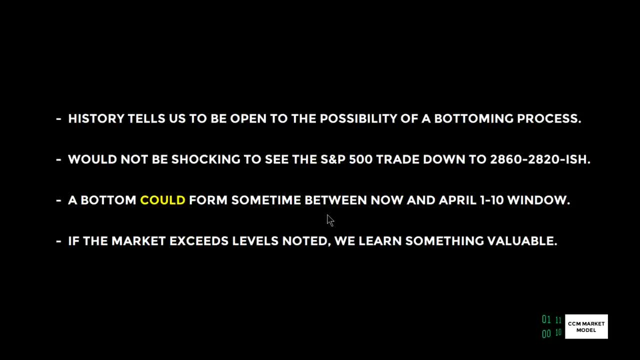 Based on the historical cases we just went over, a bottom could form Sometime between now- it's possible it's already in place- or it could form sometime between April 1st and April 10th. That's a median to average window, meaning it could happen sooner, or it could happen later, or it could happen not at all. 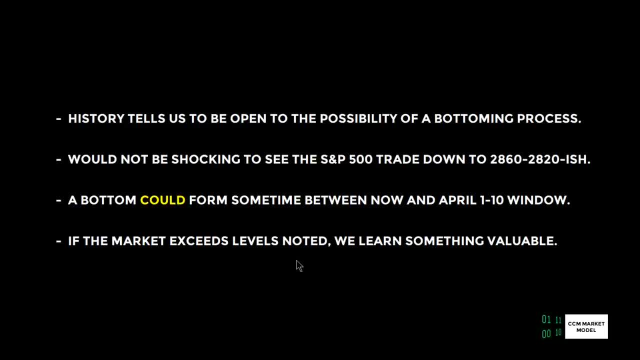 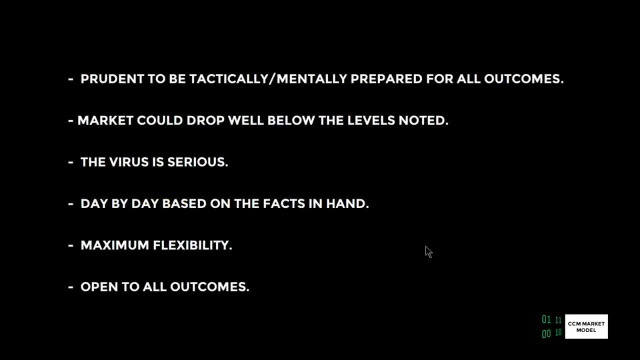 The studies are still valuable if the market exceeds the levels because it tells us that we're moving off of the base case. For all of us, It's prudent to be tactically and mentally prepared for all outcomes, And that applies every single day of the week. That's nothing new. 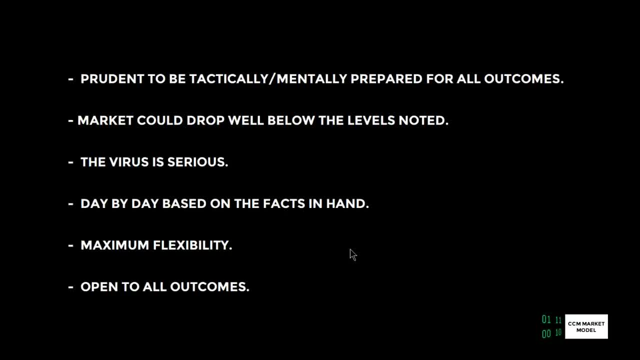 And, as we've said many times in these videos, we're not forecasting. The charts can't predict the future. They help us assess probabilities, And thus it is well within the realm of reason that the market could drop well below the levels we just discussed. 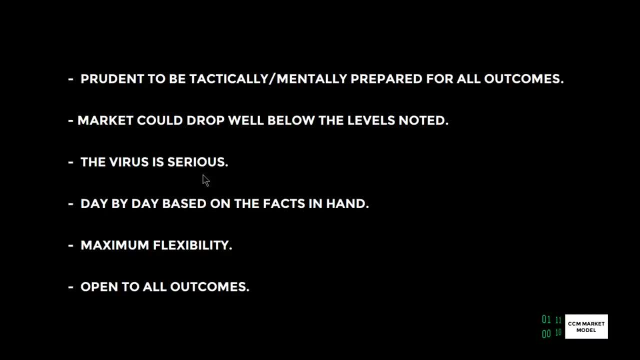 And, as we have said many times, the virus is serious. That's not even debatable. And the only way any of this works is if we take it day by day, based on the facts in hand, and we remain open to all outcomes. 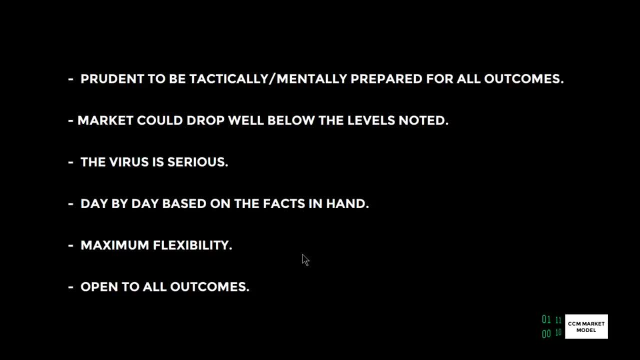 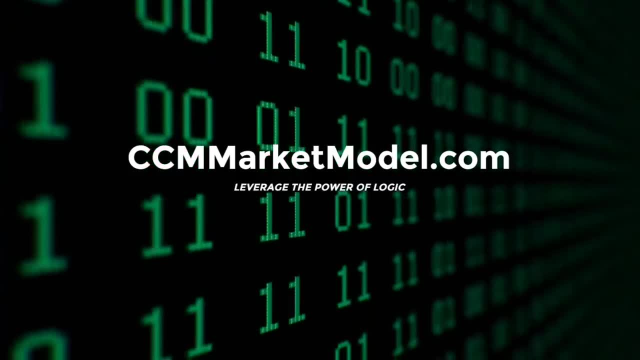 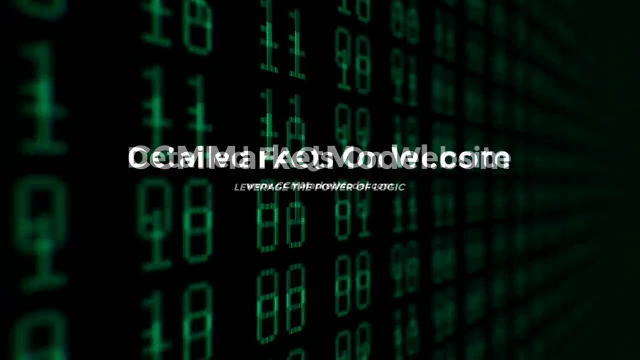 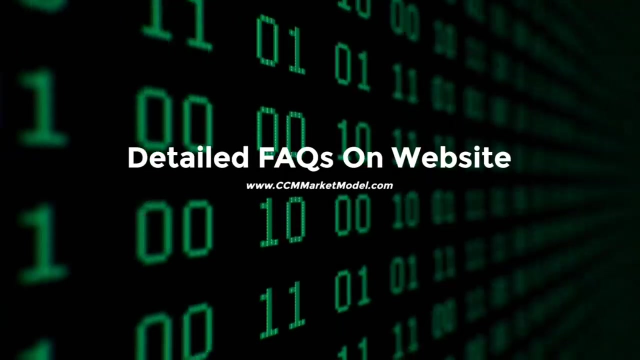 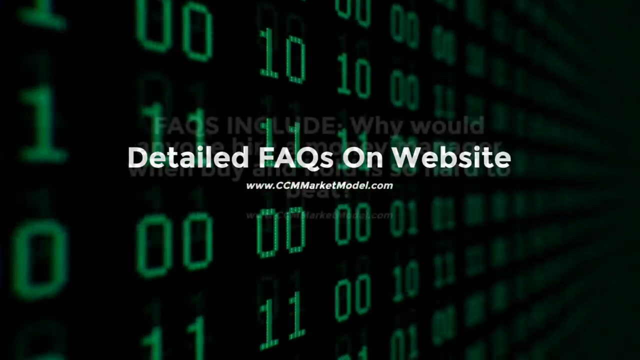 And we head into next week and every week with that flexible, unbiased and open mind. The material in this video has no regard to the specific investment objectives, financial situation or particular needs of any viewer. This video is presented solely for informational purposes and is not to be construed as a solicitation or an offer to buy or sell any securities or any related financial instruments, nor should any of its content be taken as investment advice. 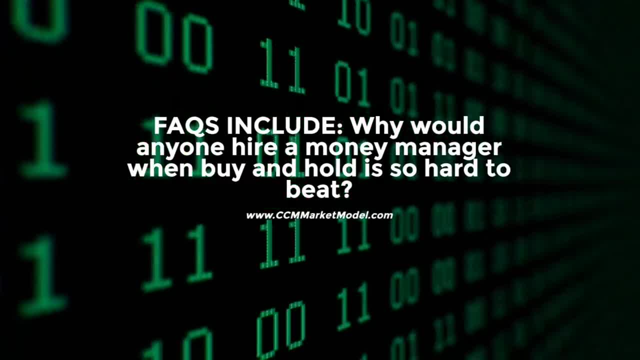 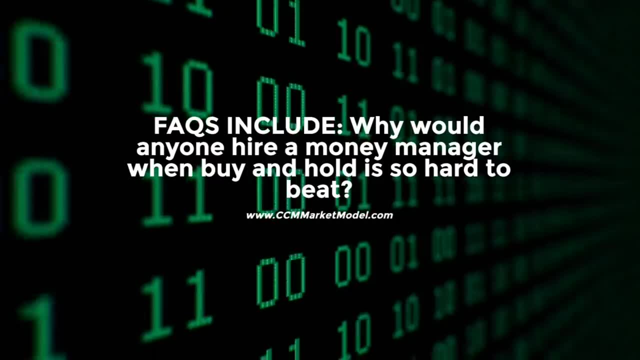 Any opinions expressed in this video are subject to change without notice, and Shavako Capital Management LLC or CCM, is not under any obligation to update or keep current the information contained herein. CCM and its respective officers and associates are available for discussion at cchavacocom. 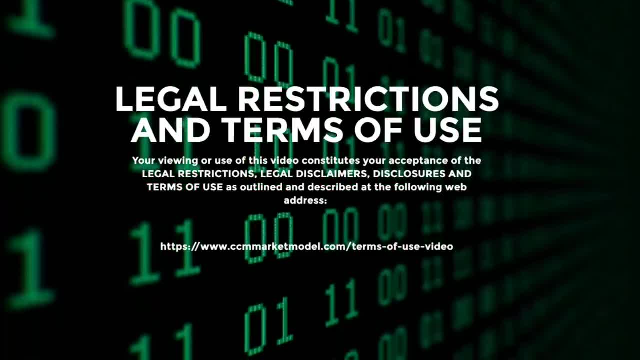 CCM and its respective officers and associates are available for discussion at cchavacocom. CCM and its respective officers and associates are available for discussion at cchavacocom. or clients may have an interest in the securities or derivatives of any entities referred to in this. 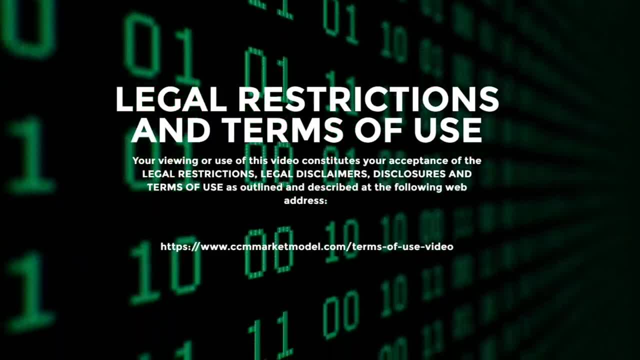 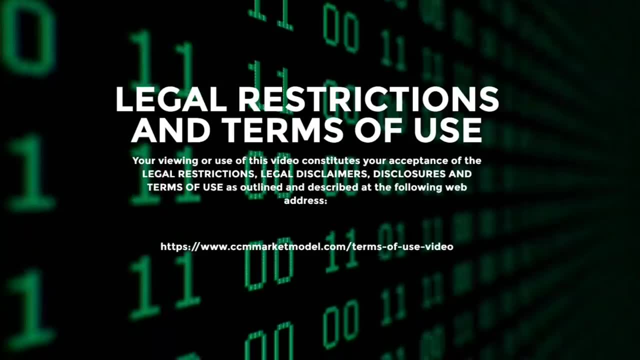 material. CCM accepts no liability whatsoever for any loss or damage of any kind arising out of the use of all or any part of this material. We recommend that you consult with a licensed and qualified professional before making any investment decision.